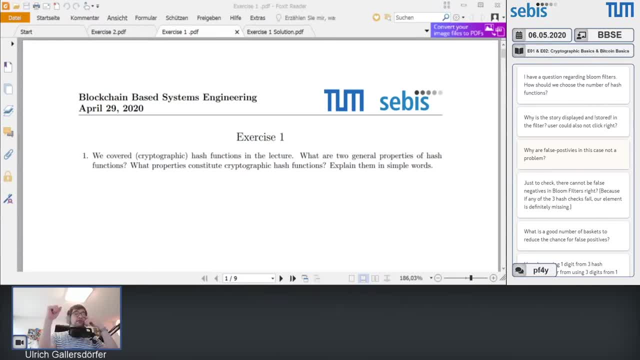 If only the hash of x is given. So you're not able to calculate x out of the hash of it. The second pre-image resistance is a little bit similar, So it's impossible to find a second x if x and hash of x are given. 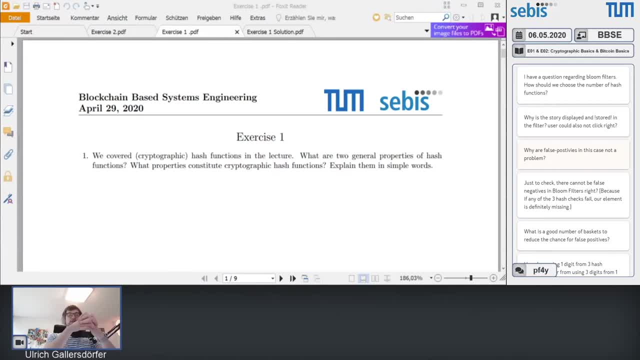 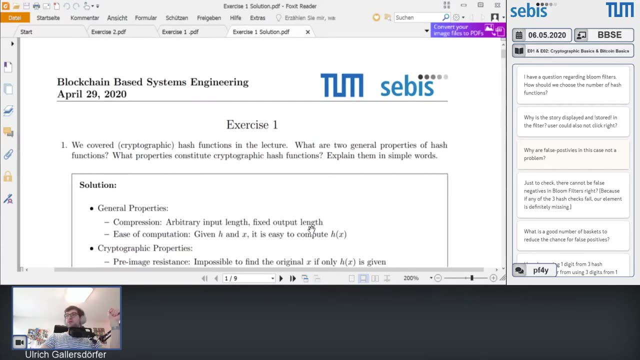 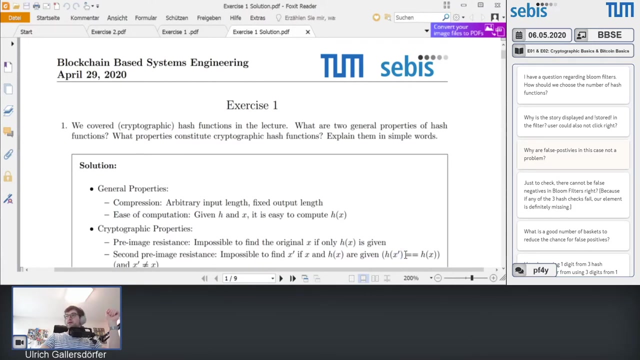 And you want now to hold to have two properties. So these two hashes need to be equal in terms of x, The output needs to be equal, but the input needs to be different. So you can take a look here. That's the definition here. So we have this second x, The hash of 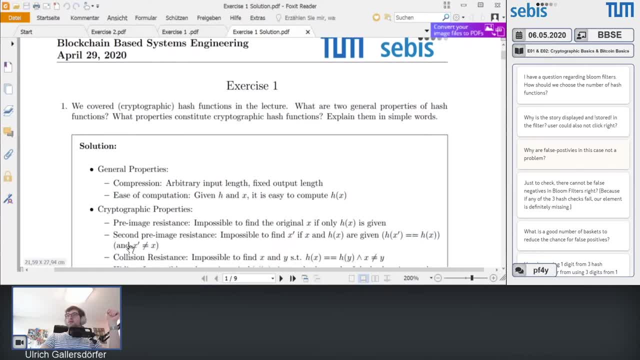 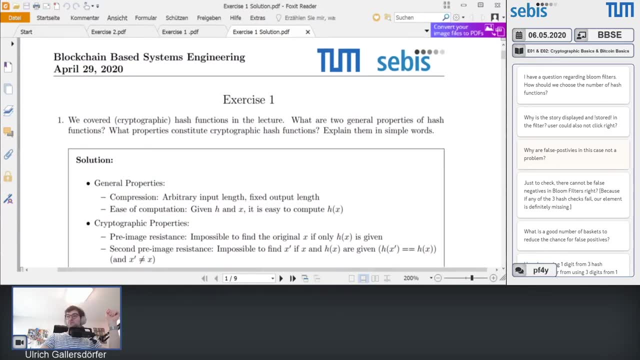 the second x needs to be equal to the first x, without them being not identical here. Then the third property is collision resistance. It's impossible to find x and y such that x and y, the hashes of them, are equal, but without them being identical. So also here. 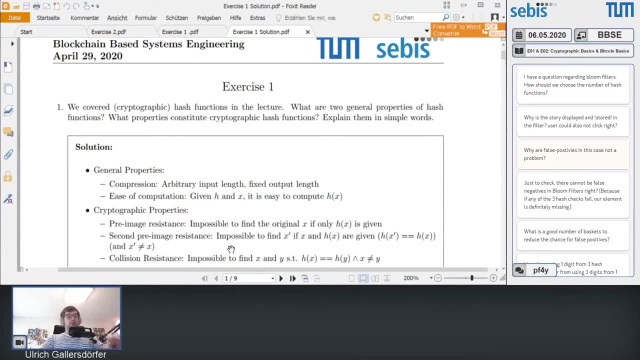 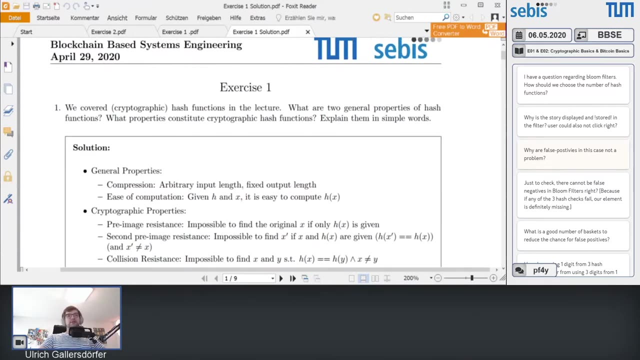 collision resistance- very straightforward property. We also discussed last week a lot about the difference between collision resistance and secondary pre-image resistance, So we're going to go further into that. And also the third property: hiding when it's impossible to determine x and then hash. 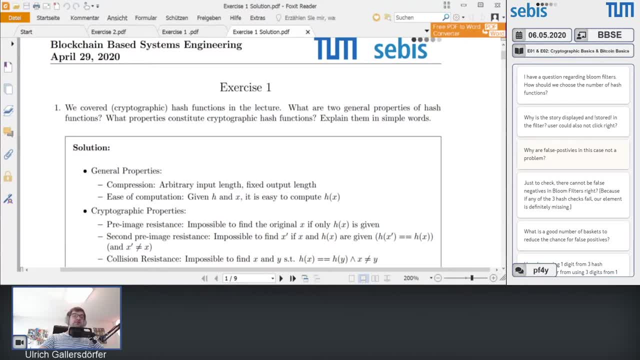 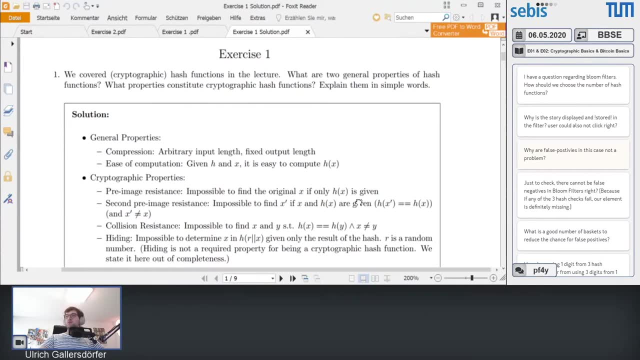 where it's basically salted with an additional value, r, And this r is a random number And yeah, so you can see also the solution here If you. we also upload the solutions online, so no worries about that. Okay, Very good, Let's continue to the next one. The next question is a little bit harder. 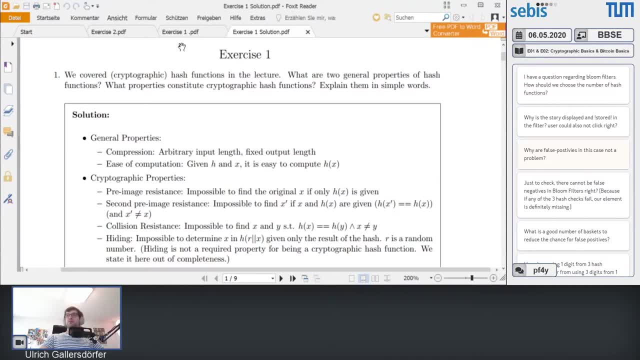 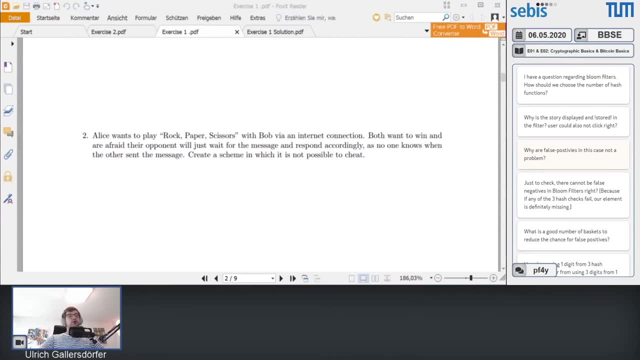 Alice wants to play rock paper scissors with Bob via an internet connection, So it's that one And both want to win and are afraid their opponent will just wait for the message and respond accordingly, as no one knows when the other sent the message. Create a scheme. 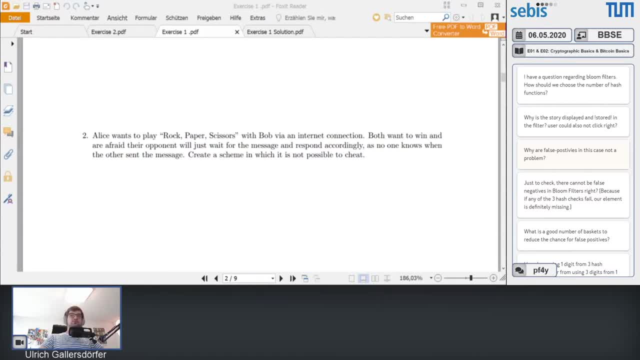 in which it is not possible To cheat. So now it's again time for people from zoom. Maybe you can share your screen. Maybe you can discuss a little bit about how you would solve this issue. Okay, Yeah, Yeah, Sure, So you're now on the stream and you can talk to all of them. 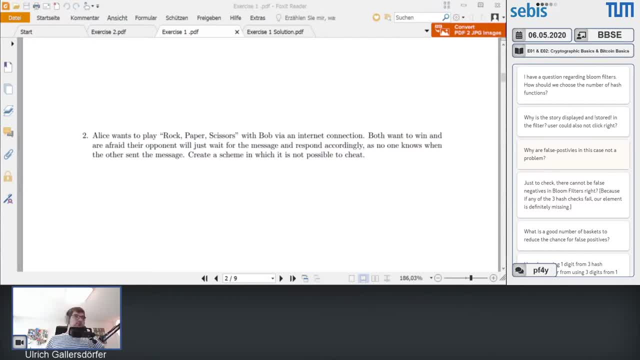 Okay, Well then I have to mute the stream, Otherwise I hear myself: Okay, Yeah, it's always a good idea. So my idea was that you can decode the decision of rock, paper and scissor as as a number. So one is rock. 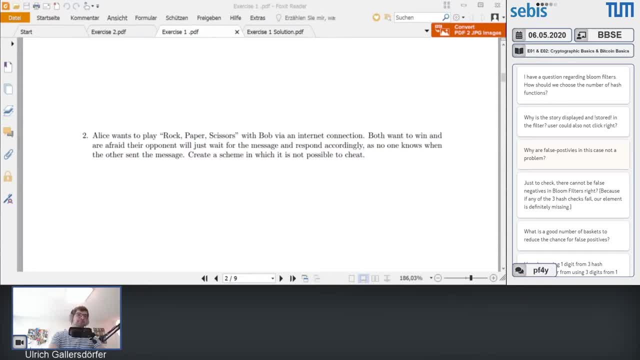 Two is paper, Three scissors: Okay, And then you have a. then you have a cryptographic hash function that is given. You can just choose that arbitrarily. And then you concatenate your decision- the rock paper scissors- with a random hash. 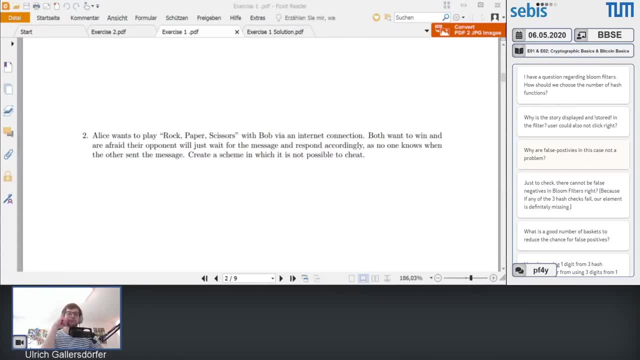 with a random number, like a large number that the other person doesn't know, Yeah, And you send the other person the results, Okay, And the result of the function, And when each person has sent the other person their hash, they reveal their decision in the random number and the person can the other person. 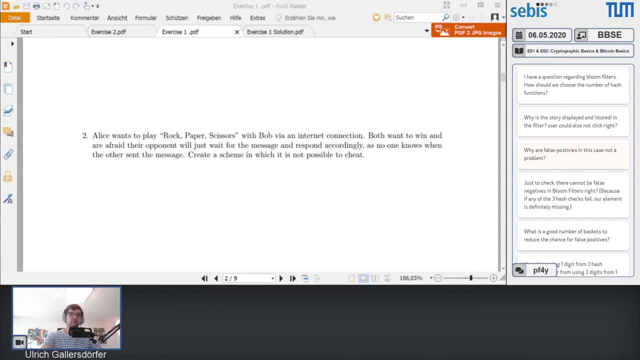 can check the decision Very good. So someone is complaining that the Zoom has a really severe echo. I don't think that's on me. I hope that's not on me, But I don't know where, where this echo would come from. 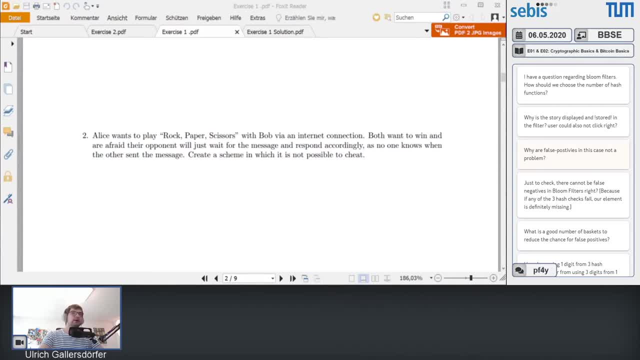 Sorry for that, Yeah, So coming back to your solution, that's exactly correct, So I'm going to display the solution on stream. So what we have here is a. we have a two way, so a commitment scheme, a commit and reveal. 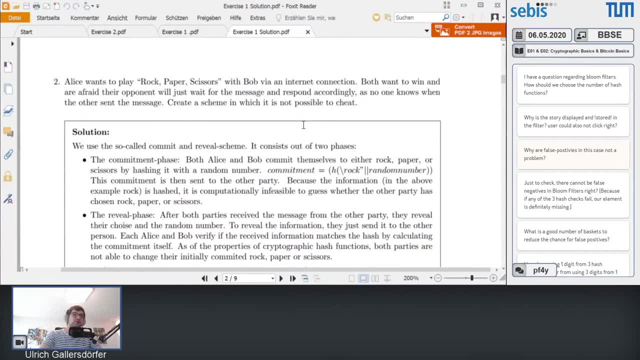 scheme. This is how this is called And this is also what we do later on, for example, in Ethereum, when we basically want to create random numbers on on the chain. So that works very well. So the commitment and reveal scheme works in two phases. 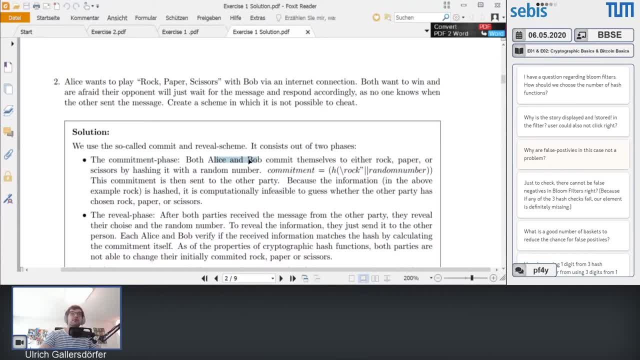 We have the commitment phase. both Alice and Bob commit themselves to either rock papers or scissors by hashing it with a random number. So what you propose in terms of putting one, two, three as the equivalent of rock paper scissors is fine. 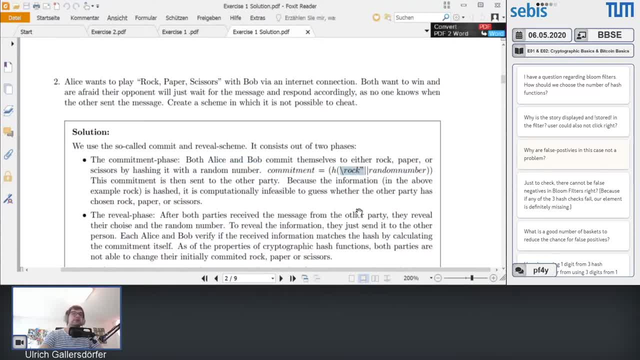 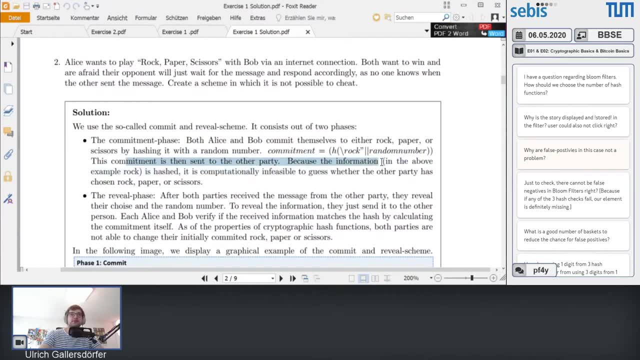 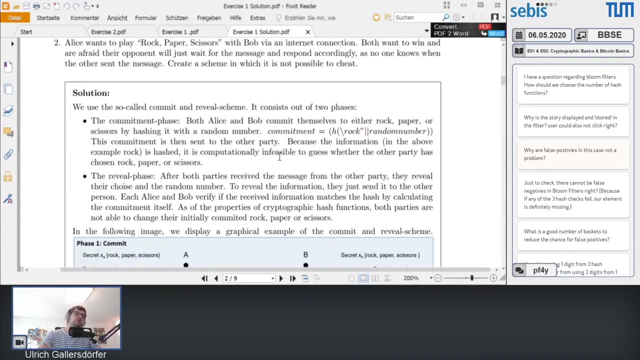 So you can also do something like that, that you basically just write it there as a string And this commitment is sent to the other parties. And because the information is hashed and hide it basically with a large random number, there is no way for the other party to understand to which value or to which to either rock. 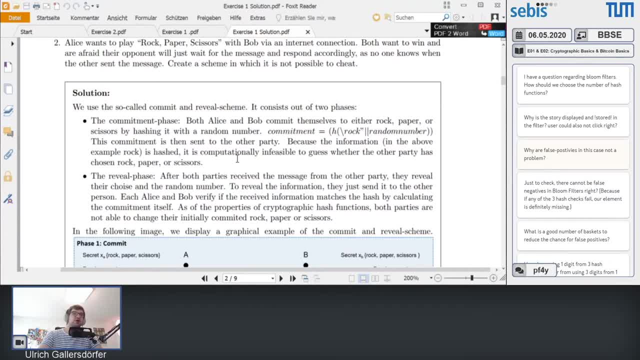 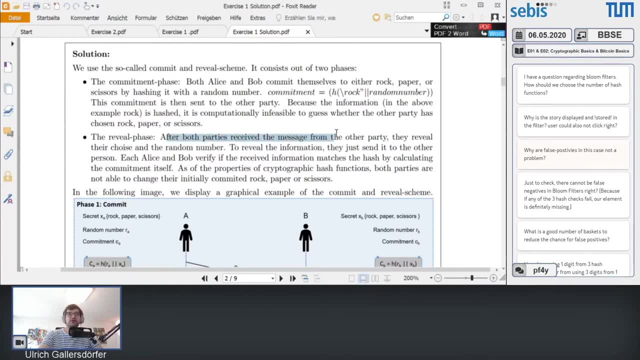 paper or scissors. The other party has committed it Itself And in the reveal phase both parties basically received the message from the other parties And now they can reveal their choice and their random number, And they sent basically this information to each other. 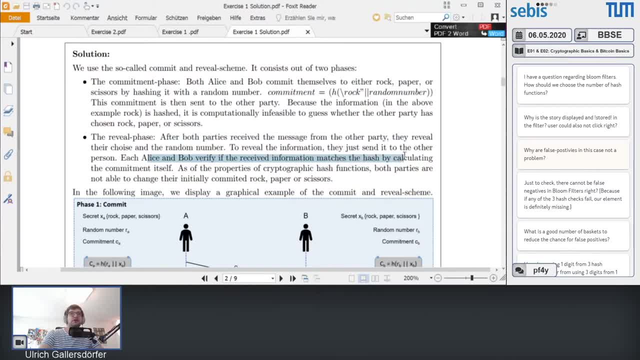 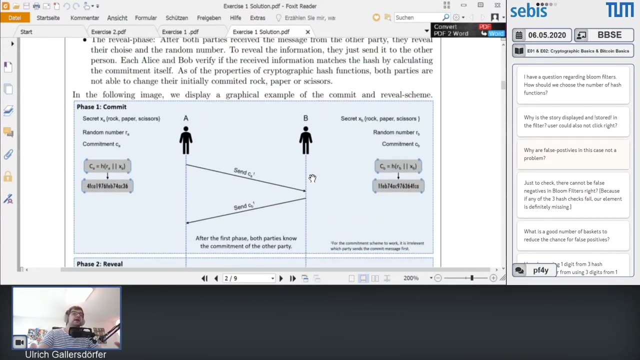 And Bob and Alice verify if the received information matches the hash by calculating the commitment itself. And as of the properties of cryptographic cash functions, both parties are not able to change. They're initially committed rock papers or scissors, So the decision they made up front is not changeable anymore because of the cryptographic. 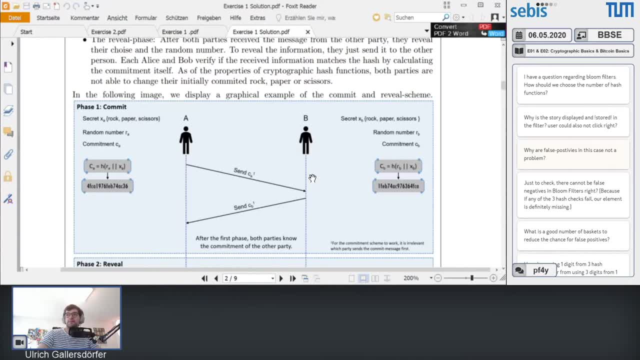 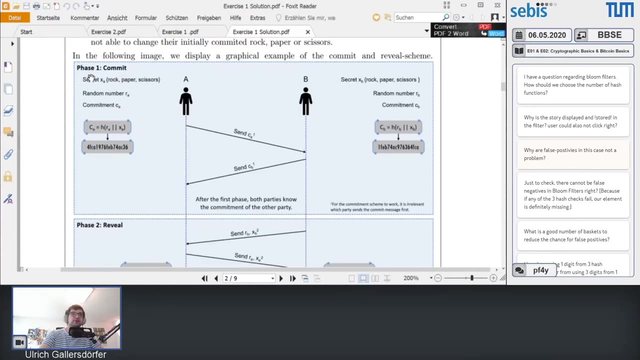 cash hash property. So you're not able- you're not really able to- to change that because of the second pre image resistance. So this is looks in detail, So this is more or less a graphical display of that. So we have the secret X, you have the secret XP. 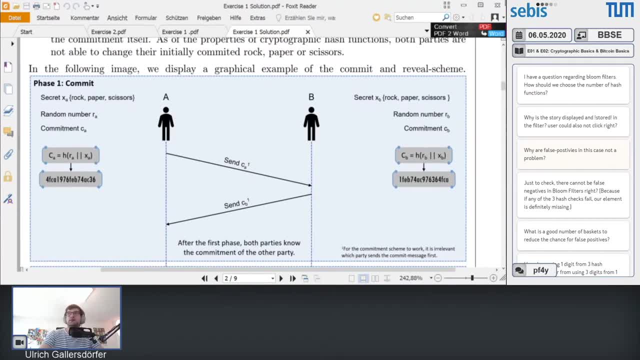 So maybe I can zoom in a little bit on that And maybe I can make it a little bit sharper. That looks good. And so we have the random number. I are a RB and we have our commitment. Our commitment is basically calculated here and here. 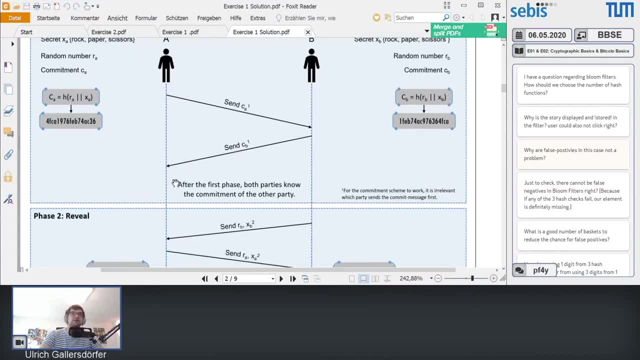 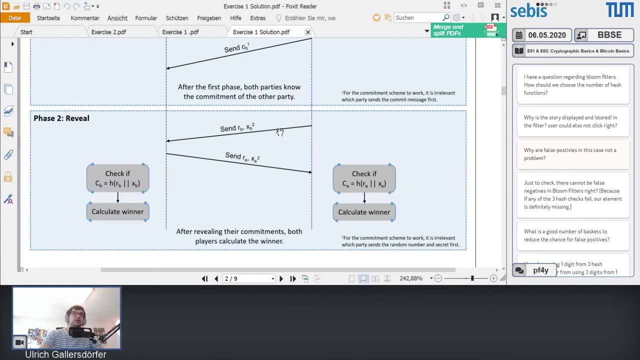 And these commitments are now sent to each other And after the first part of first phase, both parties know this, They know the commitment of the other party And now they say: OK, we now reveal our, our random number and our decision. 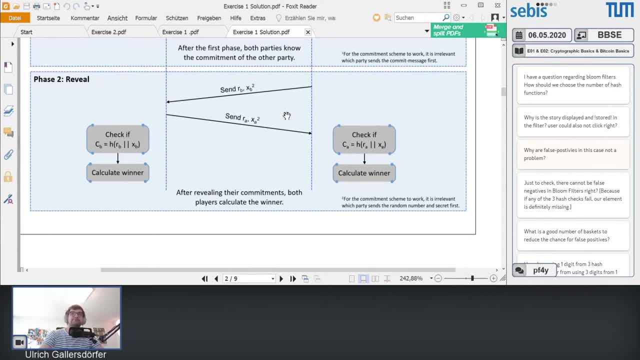 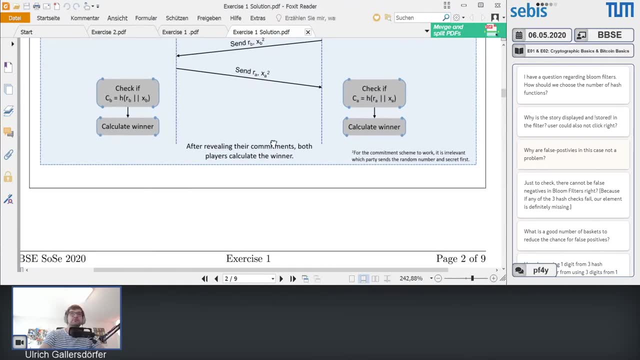 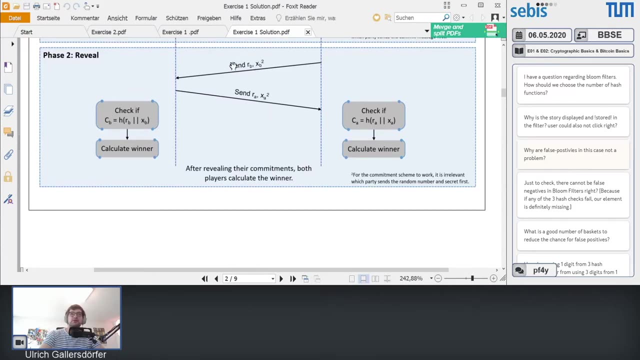 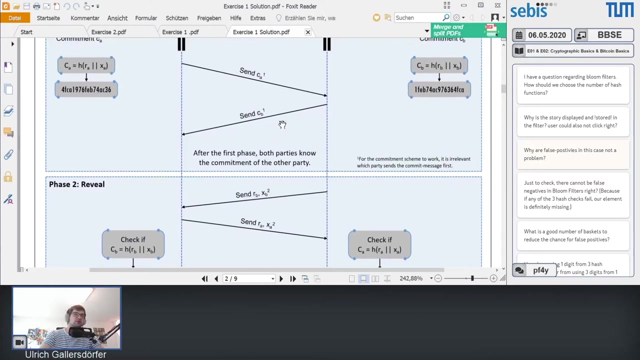 So And check if it's actually actually the correct result, And then they can calculate basically the window. Also, there It is irrelevant which party was first And It's also not important. So the the order of the sendings of the messages here is not important. 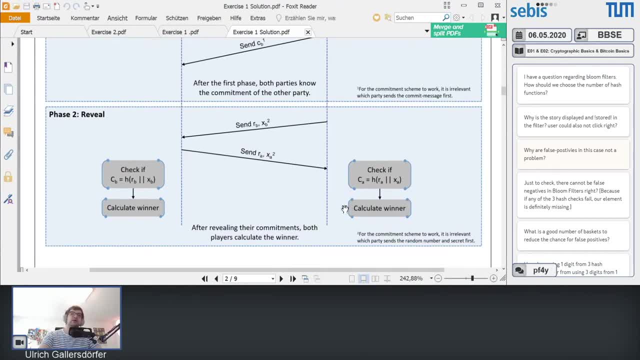 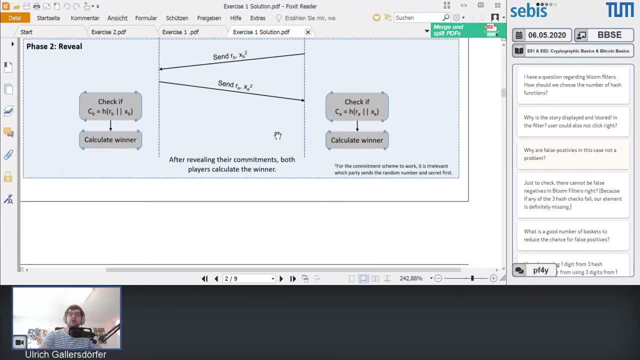 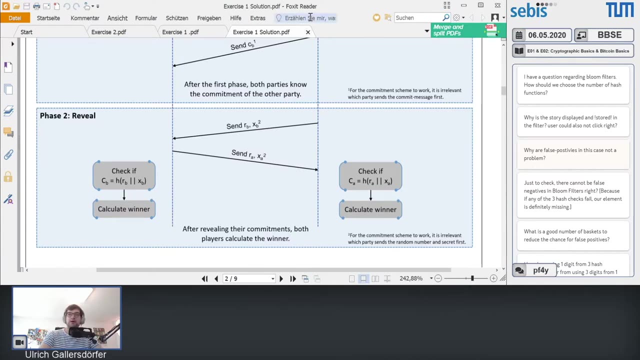 But it's in general- This is a an example- to say, OK, how could work this on chain And I would do. How would work, How would How would you do something like that? OK, We have something. We have some questions. 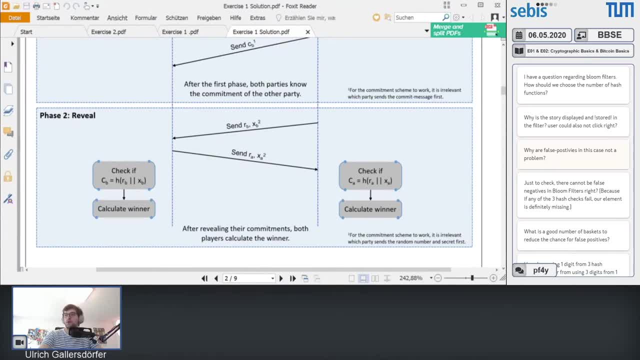 Let's take a look at them. Are there other schemes that we have to know and use? So we introduced them in the exercise And we also will cover some of these schemes in other lectures. So this is just like a little bit of a. 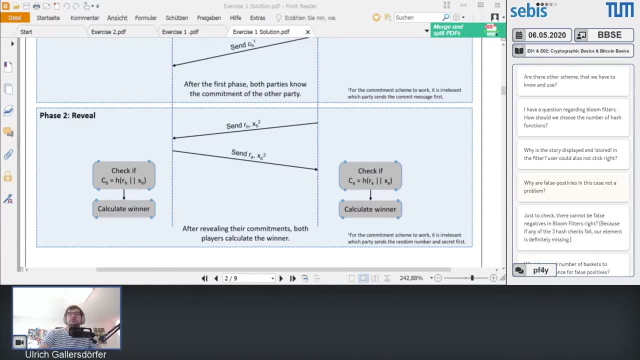 Yeah, I have a pre example, But we will introduce the most of them, or all of them we know, And Yeah, So that's definitely. You don't need to know more than that. But, Yeah, Could be some case that we use some of these schemes. 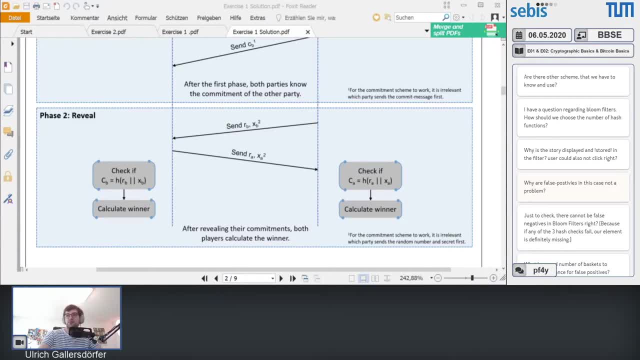 We fiddle around with them, So understand the properties, You know how to use them. That's important For Q2.. Could they send each other their choices in an encrypted file And then tell each other the key later? It is probably not the answer you're looking for. 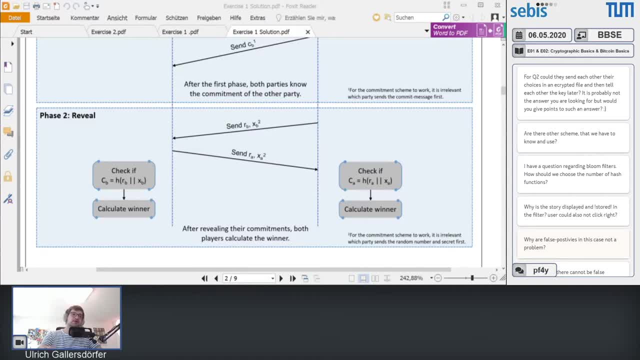 But what do you give points to such an answer? So Yeah, That's obviously a correct answer, because you can also basically encrypt data and later on reveal the key. But in The idea here is really to use what we introduce in the lecture. 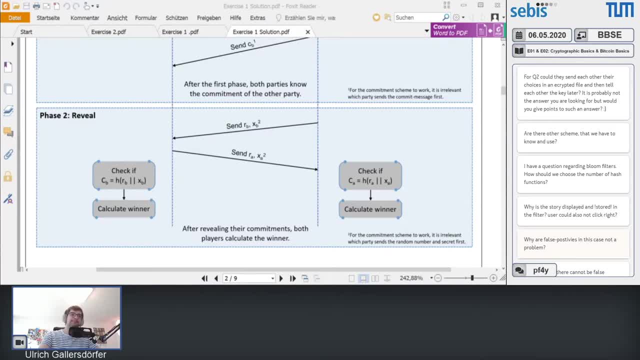 So we did not use encryption, We did not Talked about that. So it would be correct And in the exam it would be okay. Use the information suggested in the lecture, Or it is suggested to use the information in lecture. 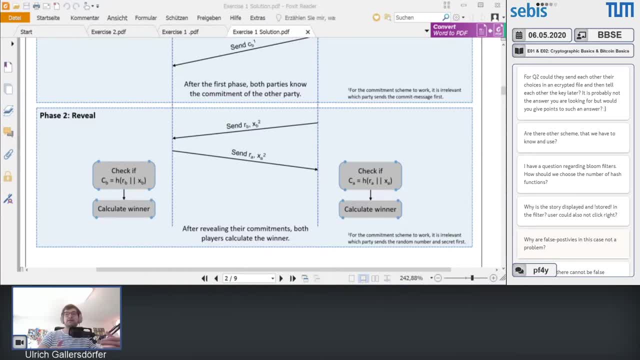 But obviously, if you are not totally off limits and if you are fine And it seems that you understood the problem and the question, Then Yeah, This would obviously Need two points. And also, I Question from And more Advanced user to atomic swaps. 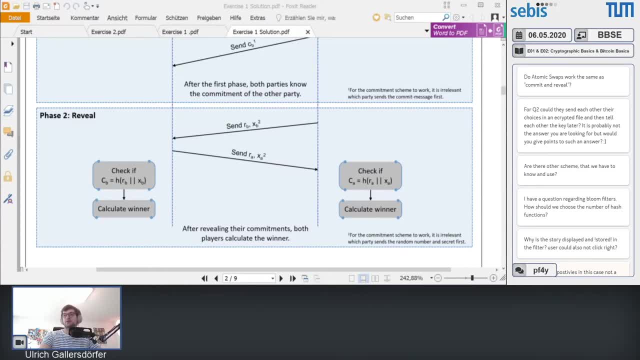 But the same as Commit and reveal. So there A community really uses Some scheme like that. So A lot of these advanced technologies like Lightning network, like These atomic swaps or Cross chain swap stuff like that, Often use something like that. 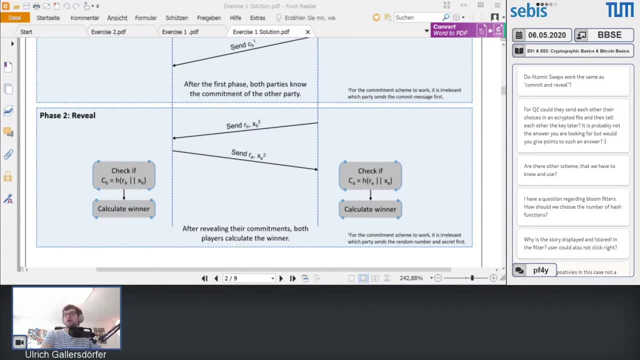 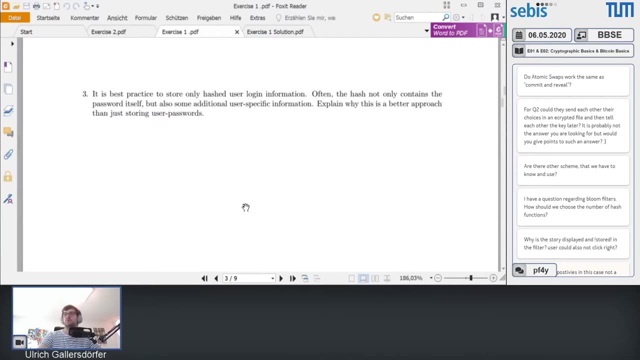 So that's, That's actually the case. Yeah, But these are Advanced technologies or advanced Protocols We do not introduce in this lecture. Okay, Let's continue to the next exercise, A Really interesting one. Not too many people also wanted to talk about that. 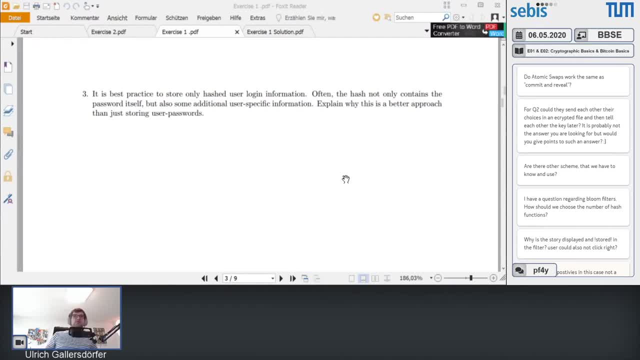 It is best practice to store only hashed user login information. Often the hash not only contains the password itself, But also some additional user specific information. Explain why this is a better approach Than just storing user passwords. So any Idea from Zoom or 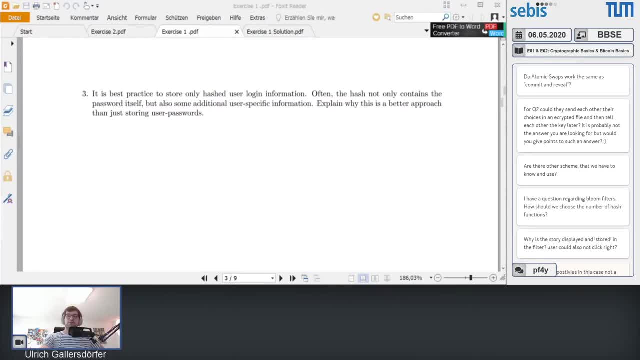 I can just go ahead. Okay, No one raises their voice And not too Important, So let's go Into that A little bit. It's actually very easy. So, When you Think about Websites, So Let's say: 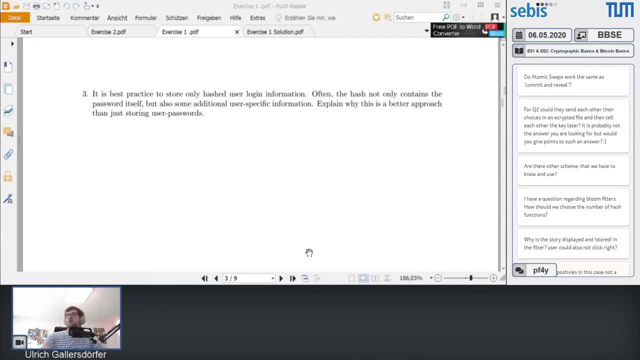 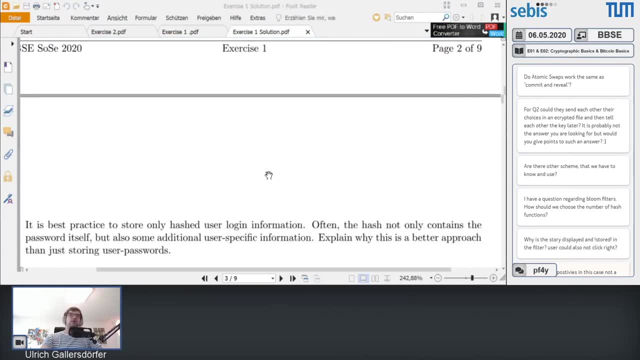 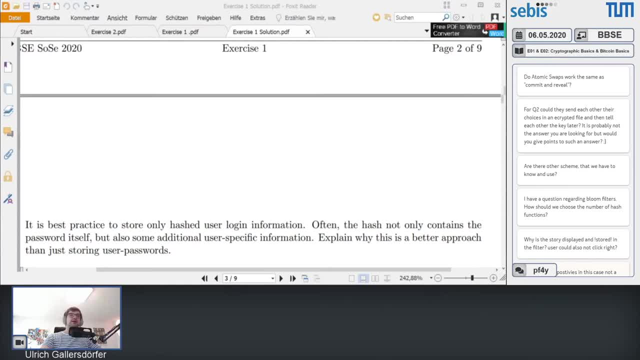 Hacked Sometimes. So If you, For example, Use WordPress Or something like that, It's Always It's A little Bit Dangerous Because It's Just Such A Popular Framework. 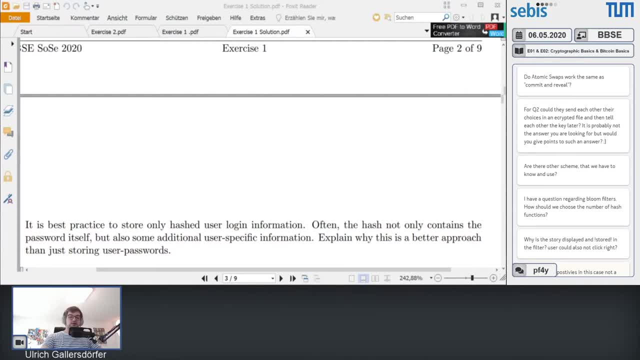 For Example, And A Lot Of Back Information Is In Their Email Addresses- Passwords, Stuff Like That And You Want To Protect Your Users. You. 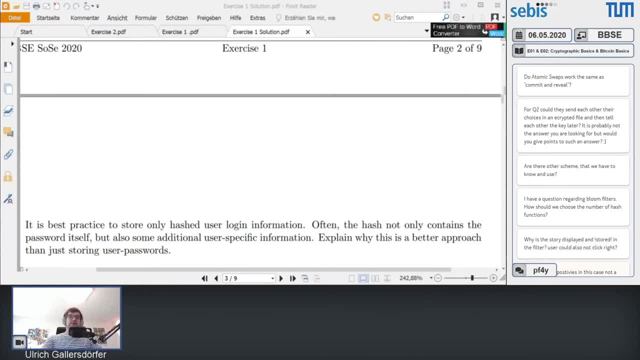 Want To Protect The Passwords Of Users, Because That's A Really Financial Yeah Systems Are Included. That's Very Important, And So You Want To. 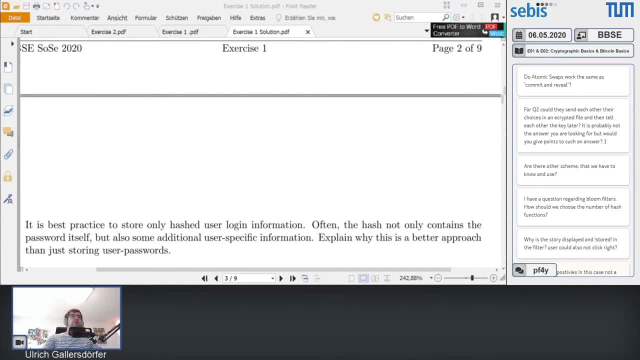 Make It As Hard As Possible For The Attacker To Obtain The Actual Password Of User, And Often It's A User Specific Information, So You 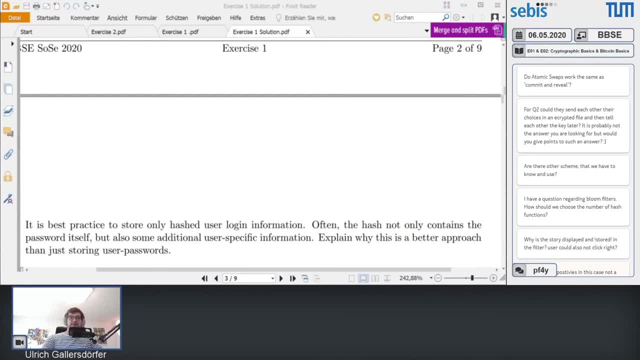 Take For Example: You Have An Additional Row, Another Column, In Your Database And This Database Basically Contains Like A Watch. And If You Do That, 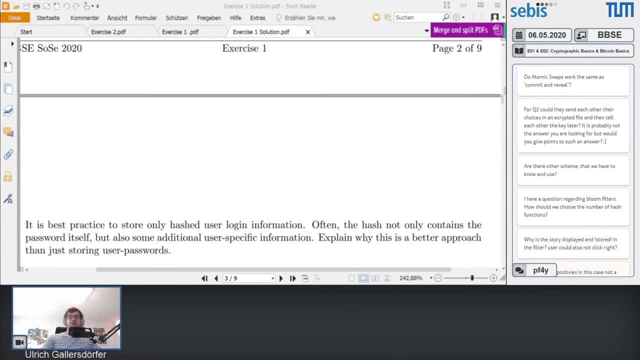 It's Better Than Just Hashing The Passwords Because On Its Own, Because If You Do That Then People Take Lookup Tables. So They Are. 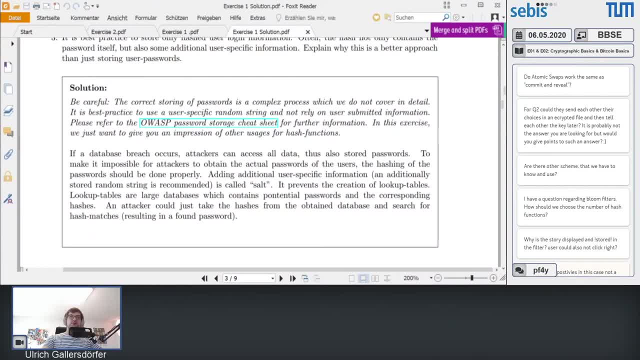 Here I Also Linked To The O V A S P Password Storage Cheat. So These Are The Experts On That Topic. They Really Understand They. 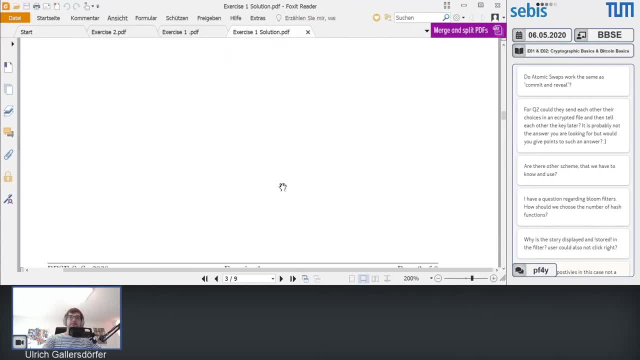 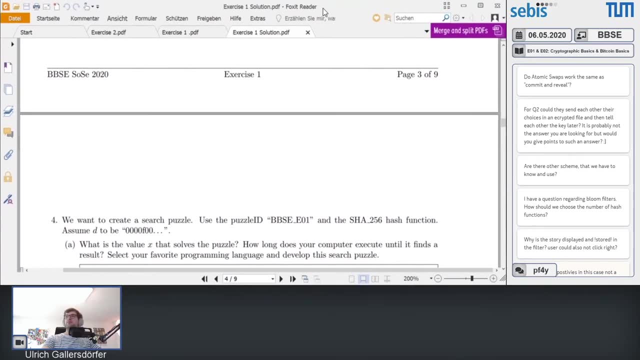 Really Know. Okay, So Let's Continue To The Next Question, And This Is, I Think, Is Where I Would Really Like To See Some, Some. 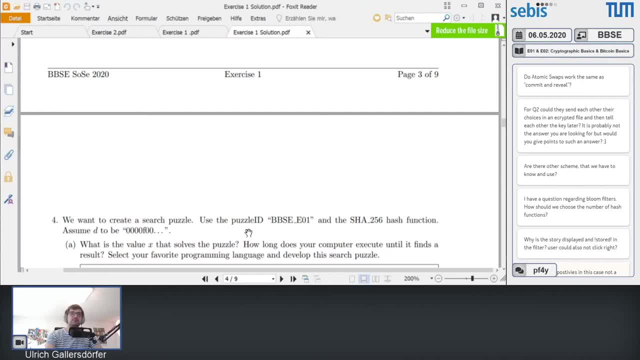 Of You, Guys, Of Your Code. Oh, Today We Are Going To To Get More The To To You Of Your Code, And To Get More. 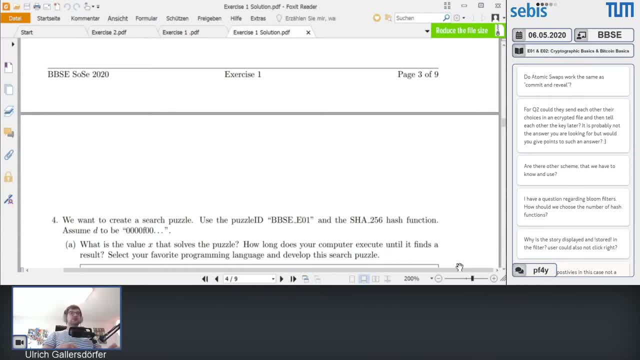 Of Your Code To Your Code Of Your. Yeah, sure, I'll put you on the stream and you can talk. Go ahead, I can share my screen. I think, Yeah, you should be allowed to do that. 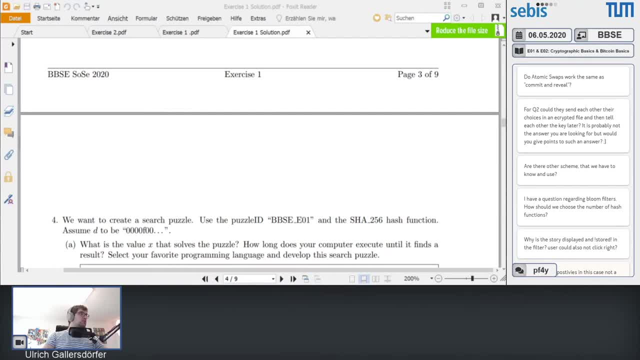 Not. yet it says you cannot share your screen without the part that's going to show you. Okay, then I need to, so now you should be able to do that, Okay. Okay, In my solution I basically use some of the information from the slide. 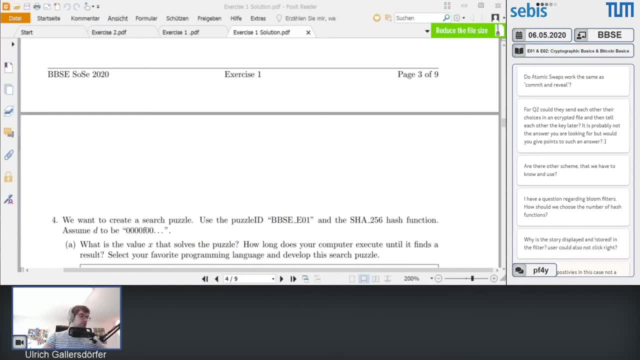 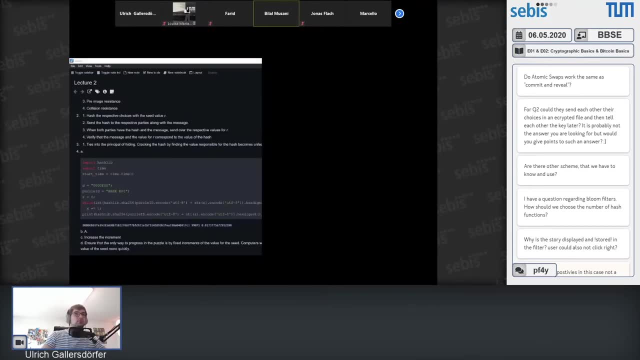 One second I'll share. I'll share the. I use the Puzzle ID and I just use the hash. Can you zoom a little bit on that, Because I only see the window. it's quite small. A little bit Okay. 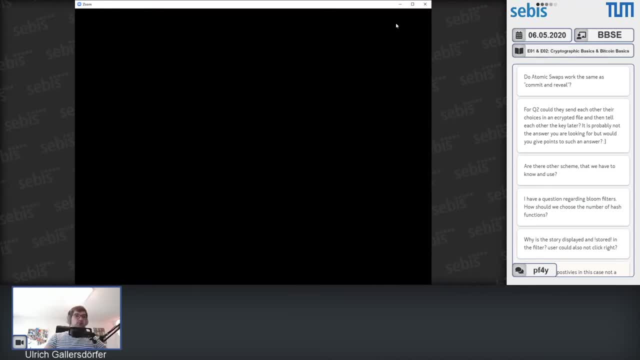 Okay, Okay, Okay, Okay Okay, Let me really watch. I don't want to show my faces. Okay, Okay, Okay, I can split the screen now. I don't want to use the distributor lights. Try to click on the other screen. 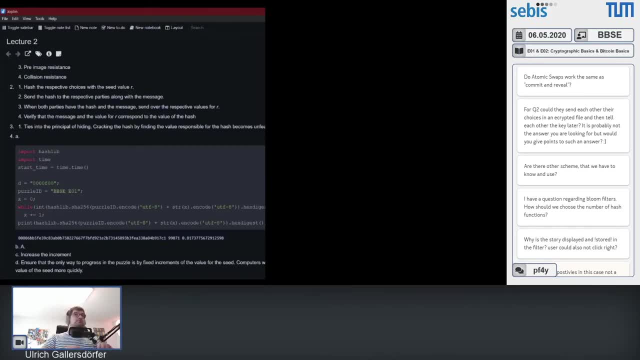 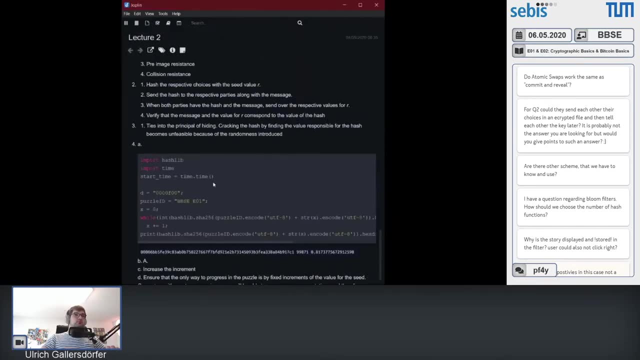 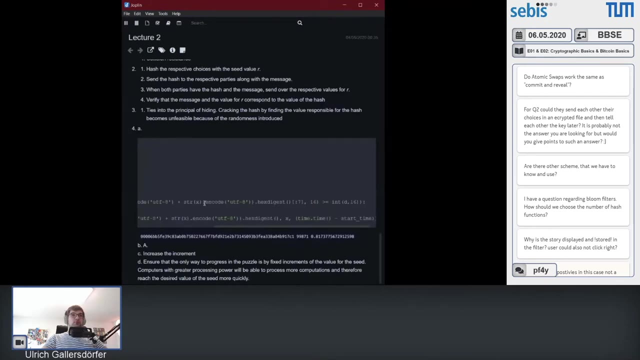 Okay, Okay, Are you listening to the person? Sorry, we can hear you. Sorry, it's too noisy right now. the hash left function from python and i just complete the hex hex digest and just try to find the first value that's lower than the provided d. i just 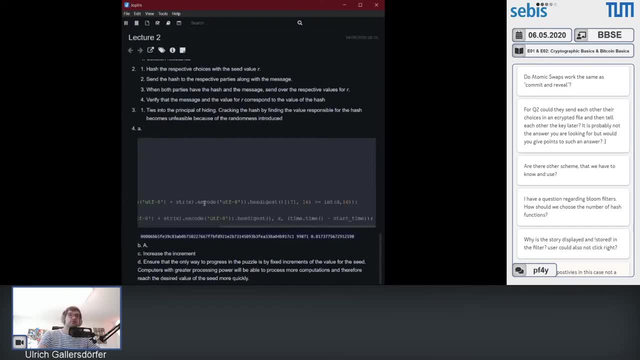 how did you um, how did you compare or how did you um? so i split it based on the first seven digits, okay, and you treated the string as hexadecimal and compared it to the d. yes, yeah, very good. and what is your result? um, i think you can see it just below the. 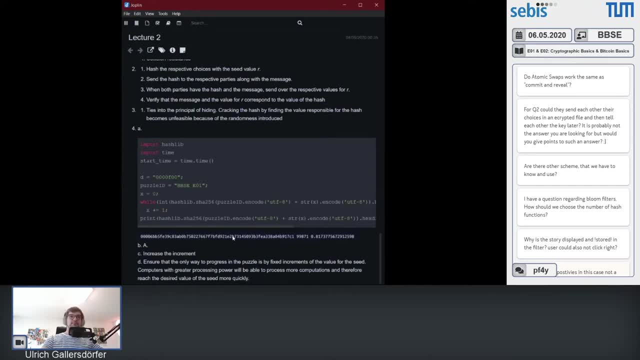 the code is basically um it. the value of x is 99 871. okay, 0.81 seconds. that's interesting, because i found another number there. the hash is um. the hash you can see it's yeah, um, it's quite, quite so that's definitely. 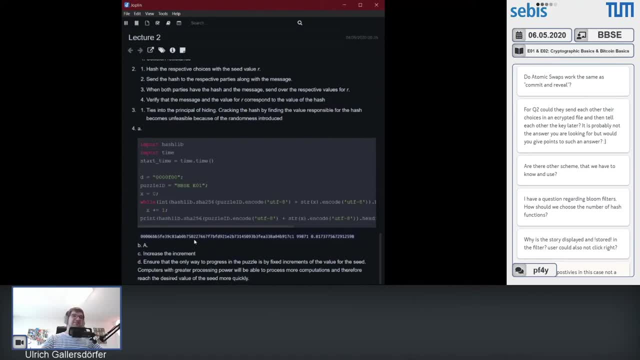 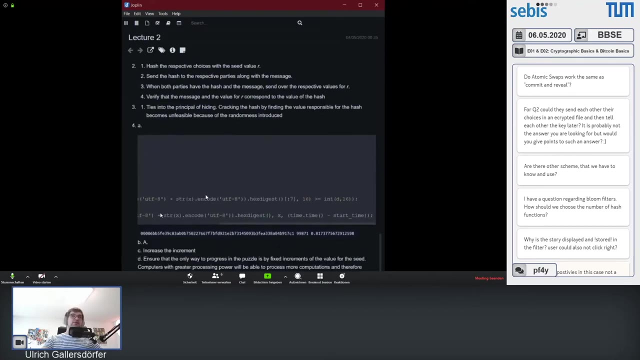 a correct solution. i have a. i have a different solution and i think the reason for that is because in your um you say you encode the puzzle idea as utf-8 and i'm not sure how that um turns out in the um. how you did not? you used a blank instead of a under, under, under, underline. 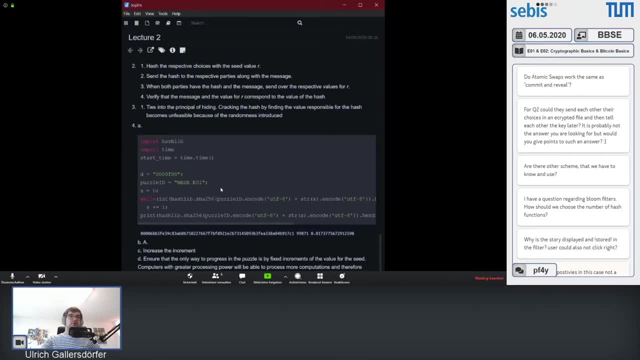 the puzzle id. that could be the case. that could be the reason for it, um, but i have, i have, so, so it's, it's correctly programmed and you did it actually right. i hoped for someone, um, for a small mistake, but i will show you a common mistake, or we'll talk a little bit about that, but that seems very good. i also will show my. 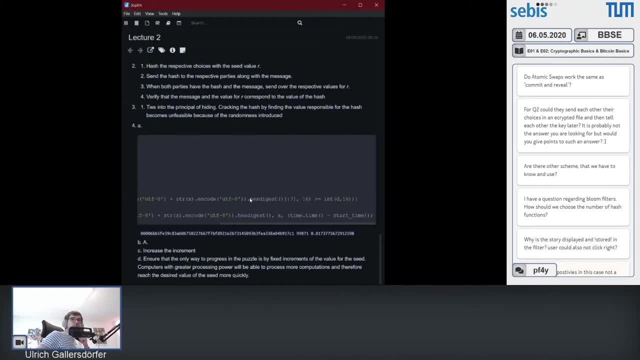 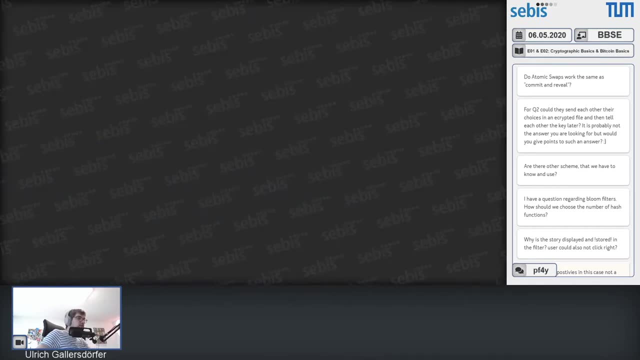 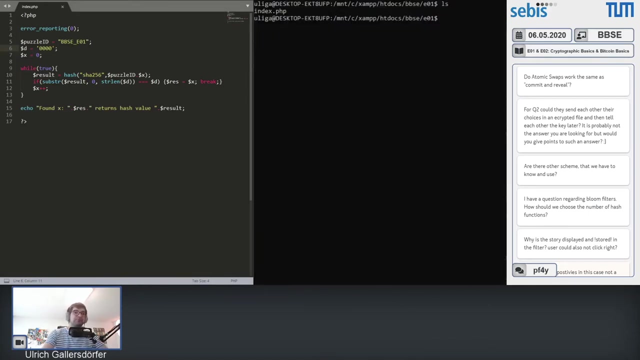 sus code in a second. um, okay, thank you very much. let's turn this off very good, okay? so i what i have is a. i'll share my solution here and this is my console here, so i will walk you through that so that you get an understanding of what is going on there. 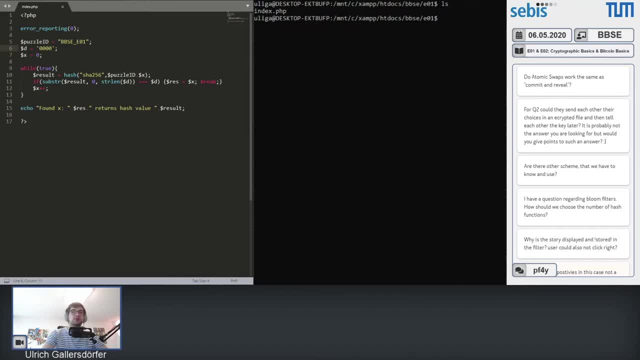 i have to find my data and there it is exactly. so we have our um, so i program in php, um, so i just have to do that um, and you might wonder what is wrong with this guy. and um, that's the first programming language i learned in my life, so that's also the i spent the most. 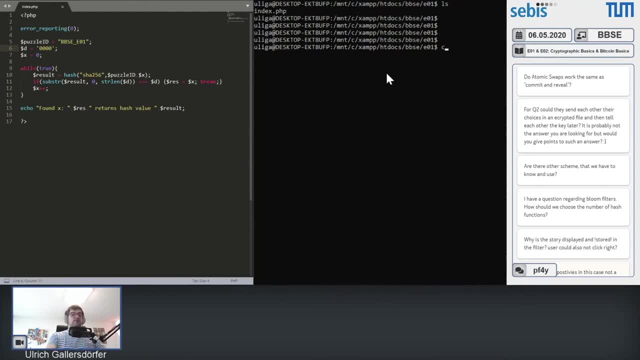 time with, and therefore it's the easiest to do it for me, um, but you can do it with every other um, every other language as well, so no harm there. um. so what you see here is um. obviously, we set the error reporting to zero, so that's very important, um, if your real program just disable the errors and 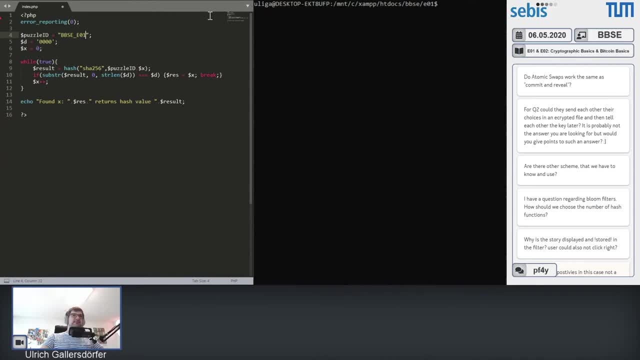 works fine. I defined the puzzle ID, so bbse, under slash e01.. I defined the difficulty d, so four zeros. I defined x starting with a zero, And I have a while true loop which basically does the following: So we calculate the hash, So we use SHA-256. 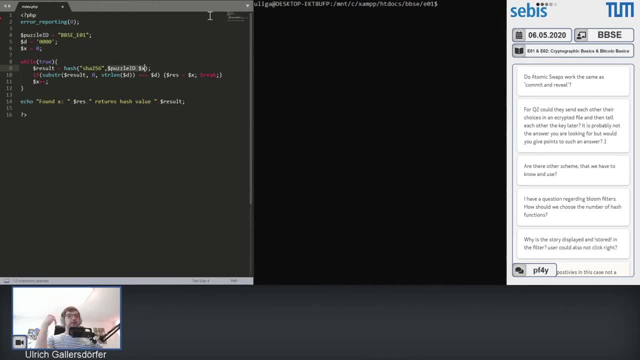 of this thing. So we take the puzzle ID, in this case bbse, e01, and the x. So the x is here like this one, And this concatenated is hashed, And now we do some cruel- it's really cruel- comparison. So what we do is- and your student did it correctly because he took 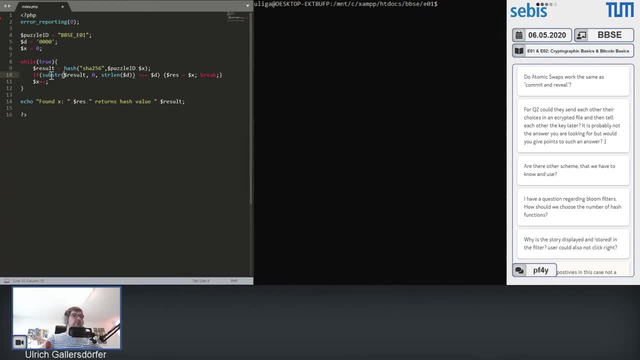 the number the hash interpreted as a hexadecimal number and took that as a comparison. I made it a little easier for myself because I said, okay, I don't care about hexadecimal here right now And I just want to look if the first 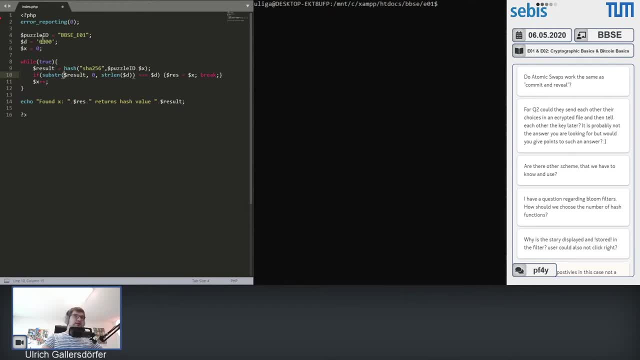 four characters start with a zero, because that's what we need here, And what we do is we generate a substring out of this result, starting from character zero for the length of our difficulty. So this string length basically returns four. but it's also if I would write here: 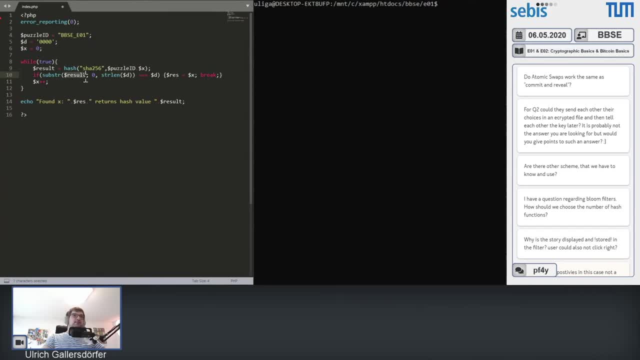 four. it's the same result And I check if, basically, this, the first four characters of our result here, is equal to d, And if that's the case, then I say okay, I define the variable res as x so that I: 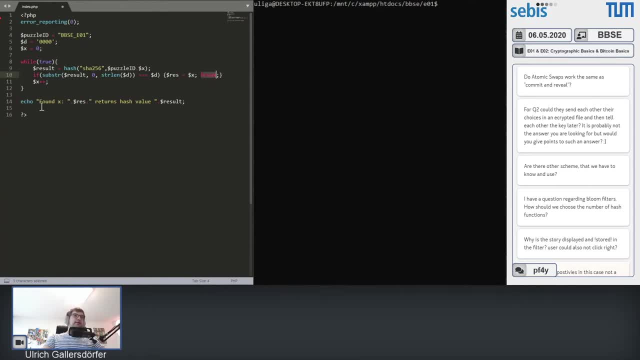 know, okay, what's going on there and I break And then I can say, okay, after that, found x, our x returns the hash value like this and that. And I can do it now here. So if I take a look, 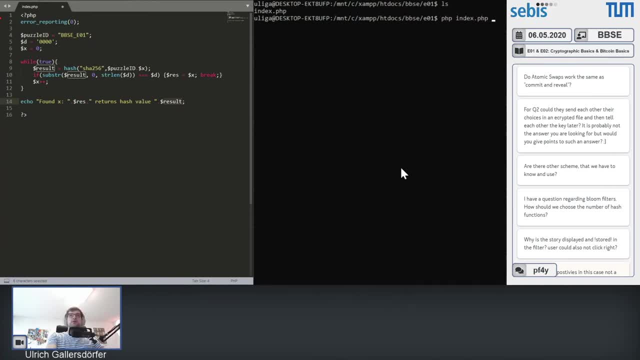 it's only the index PHP, and now I can do PHP, index PHP, and it generates for me five, seven, eight, five, two, And with that hash value. I don't know how many of you tried it, but that should be the solution for for the exercise here. I did not. 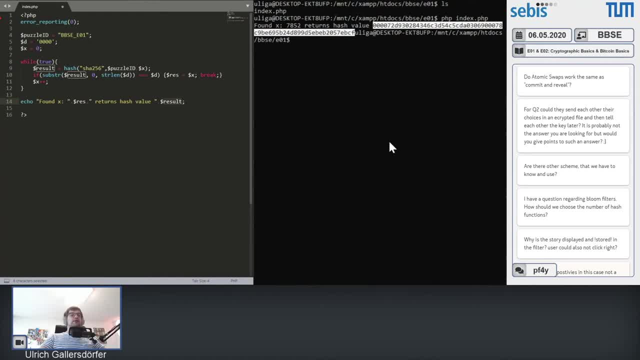 I did not try how long my computer takes and because it really depends on your machine, So also where you use it. So this is a a so-called Windows subsystem for Linux. So on my Windows machine this is like a small Linux machine where I can do all the fancy stuff. 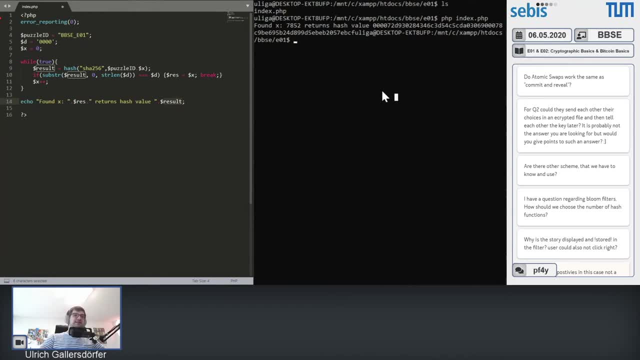 People start asking why I did not do it with Solidity. Very good question. Solidity is a programming language for Ethereum and Solidity is not made for compute intensive work, So it's it's a? it's a software or is a programming language which is used for on-chain? 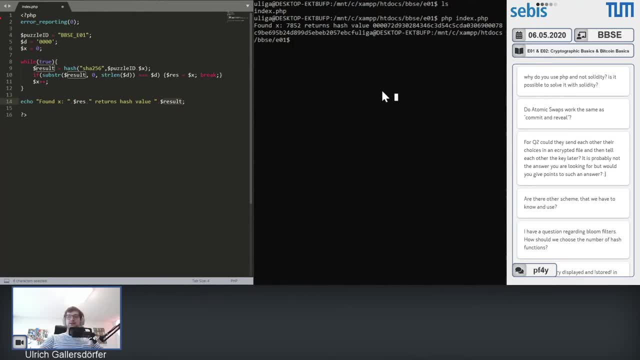 calculations, And each of these nodes in the network basically have to compute all these these steps on their own. So I do it locally on my machine. I don't have to run it in Solidity. I think it would work. It could work, but Solidity is such a slow language. 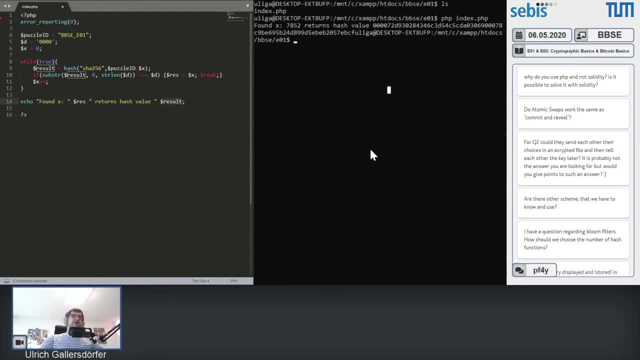 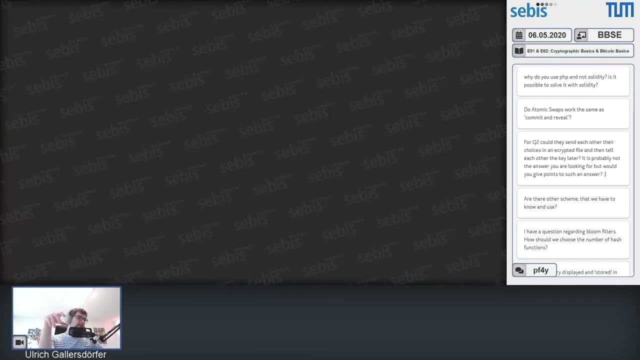 such an in performant language. So really don't use it for any heavy computation. Just use it for, for, for what you really need to do on-chain. but that's story for another day. Okay, Let's look back at the exercise So we can take a look at the solution. 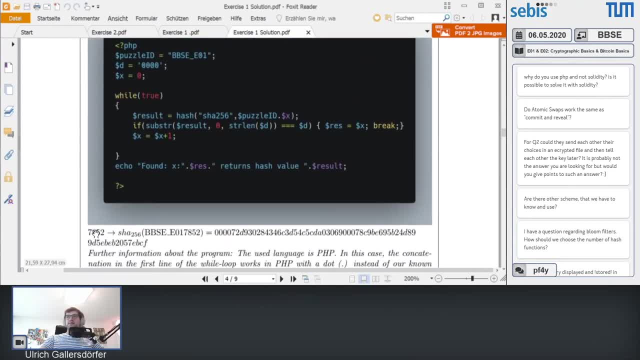 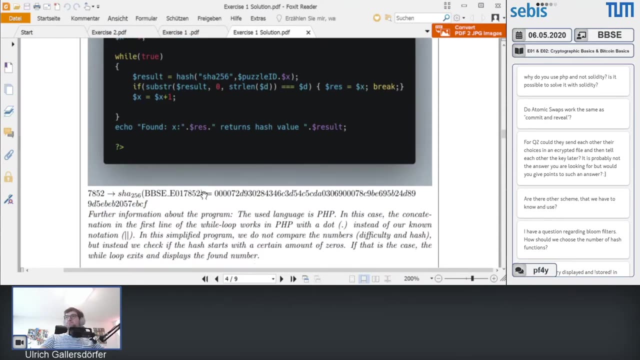 and that's the code here, And that's the result here: 7,852.. That's, that's the. that's the result here And further information about this program. So this is how PHP basically allows you to concatenate numbers, stuff like that. So the puzzle ID. 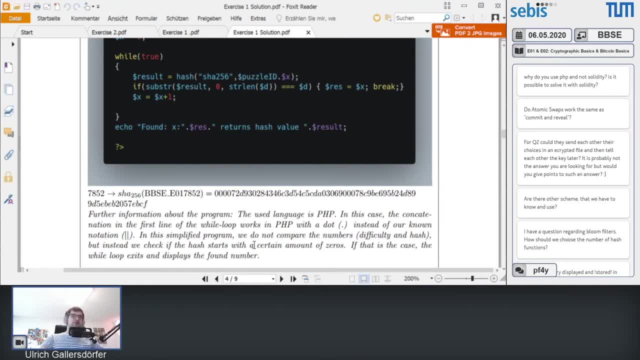 with X is concatenated just by a dot. in JavaScript, for example, you would use a plus, So, but that's, that's totally up to your, your programming language. So maybe let's talk about, let's talk a little bit about what the what the downside here is with my approach. 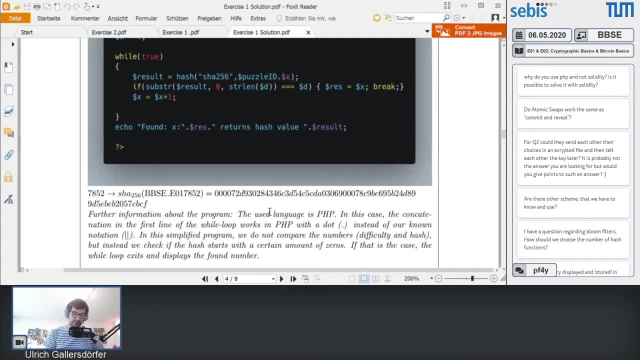 because I think it's a little bit- it's my solution- sometimes gives a little bit of a simplified idea of what's going on. Oh, the problem here is that if we look at these- um, if what? what I do is we want a hash. 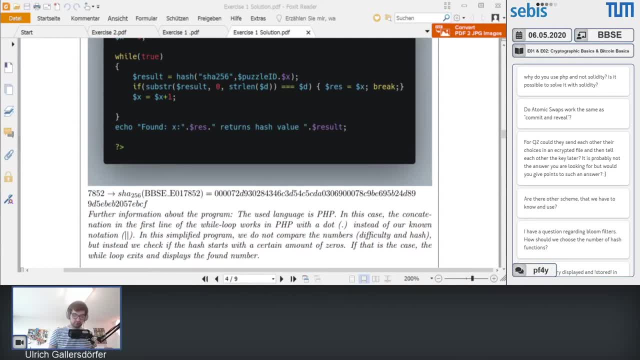 which starts with a: four, six, seven, eight, nine, 10,, 11,, 12,, 13,, 14,, 15,, 16,, 17,, 18,, 19,, 20,, 21,, 22,, 23,, 24,, 25,, 26,, 27,, 28,, 29,, 30,, 31,, 32,, 33,, 34,, 35,, 36,, 37,, 38,, 39,, 40,, 41,, 42,, 42,, 43,, 44,, 45,. 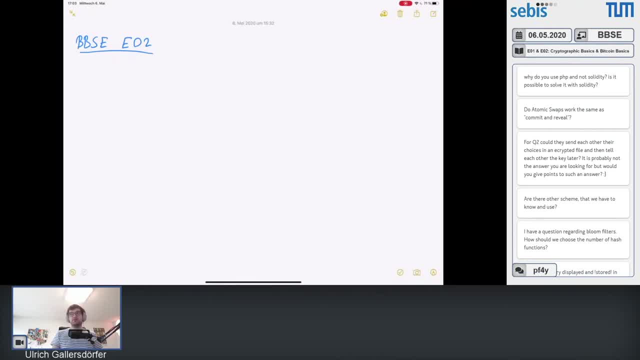 35,, 40,, 40,, 44, then the problem here is that if we look at these, if what? what I do is we want a hash which starts with four zeros And what I do is, basically, I can only allow for this hash. 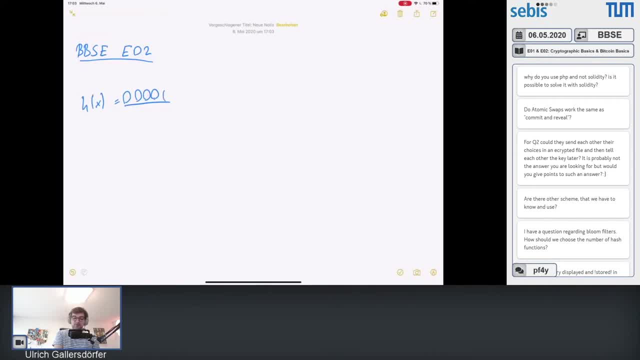 If it has to begin with something like four, four zeroes, five zeros, and it actually does not matter if you say it should start like that or it should start like that, Like it is always um. so the difficulty here between that and that is different, but between these two it's equivalent. 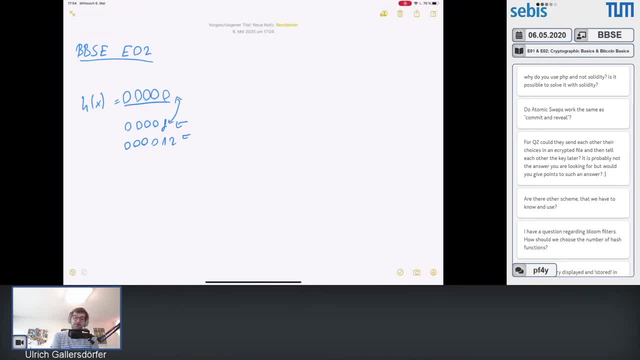 And um, if you just look at the um, at the strings here or at the beginning of the hash, then it's not totally correct. Because now, if you would do it like that, you can only um increase the difficulty and reduce the difficulty by the. 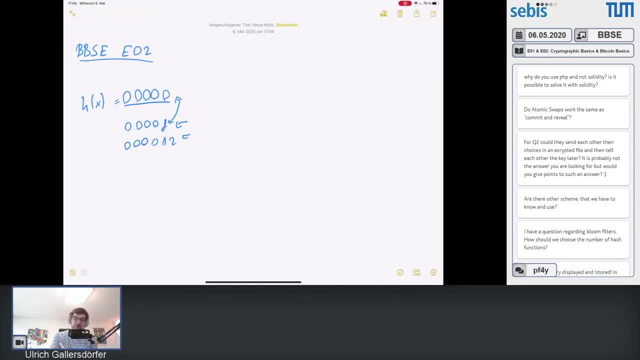 factor of um 16.. So if you would say: okay, now we have um, now we want to find four zeros um, and then we want to find five zeros. So now that's some kind of takes an amount of I don't know what, but that takes off. 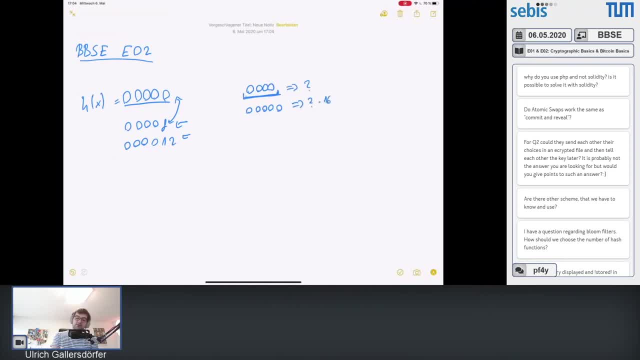 There's no, we don't know what time- 16, because, um, this additional number has to be far found there And um, so it's really important, Okay, Or um, for Bitcoin, of a blockchain, it's really important that we say: okay, we need to have something like below or equal to zero, zero, zero. 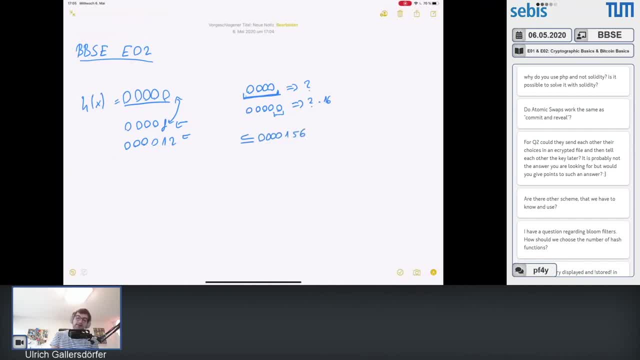 And then, for example, one, five, six, And then with that, with that approach, like really saying, like your colleague did it very good to say, okay, we need to treat it as a hexadecimal number And we really need to need to make a, a size, a comparison between these two numbers. 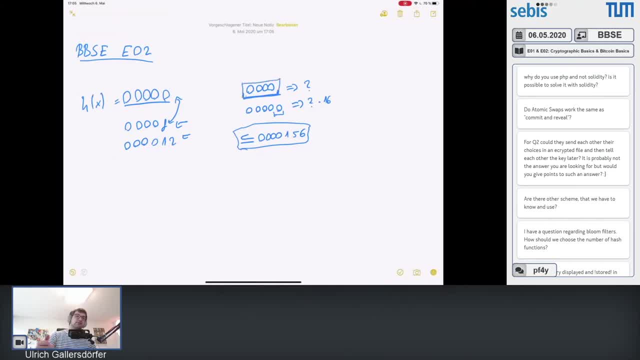 If you just say okay, the first four characters here are Relevant, or the, the, the, the, the, the leading zeros are relevant, Then you um reducing that to only these times. sixteenths, or divided by 16: difficulty. 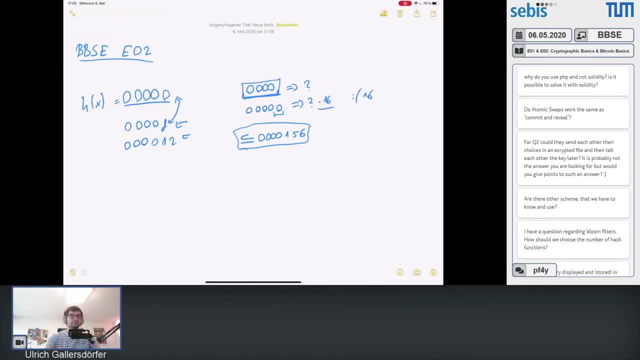 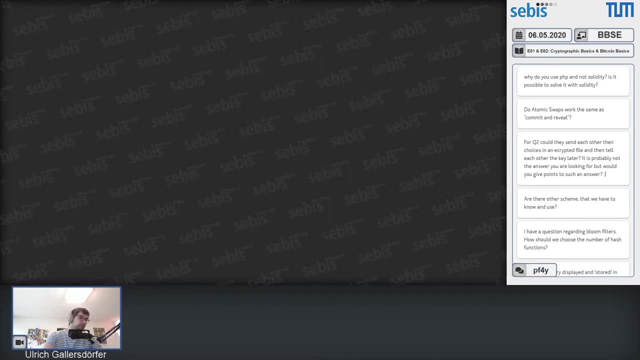 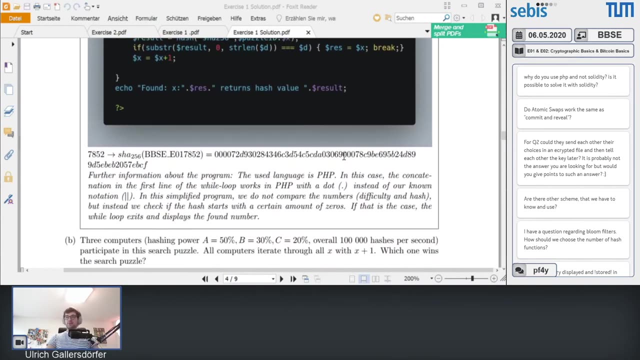 And that's not really, um, not really useful in terms of blockchain, because I- you will see later on the reason why- okay, let's continue, because, um, I'm um, exactly, So, um, I'm going a little bit. 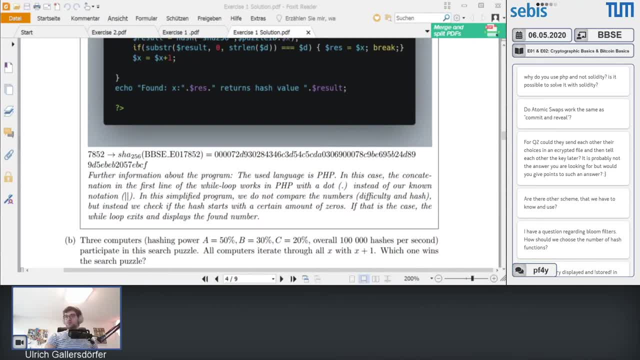 Over this now, um, I think, um, then we focus a little bit on um the uh lost, lost the parts, And um, so um, three computers. hashing power: 50%, 30%, 20%, overall 100,000 hashes per second. 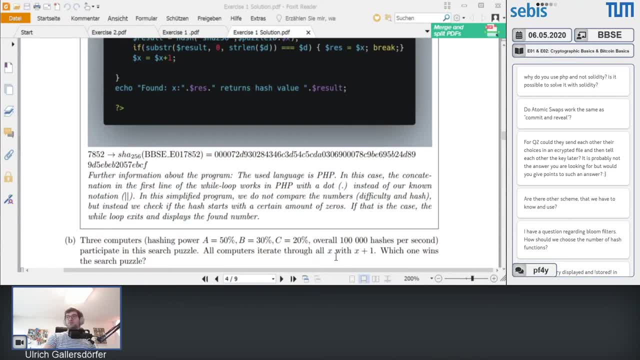 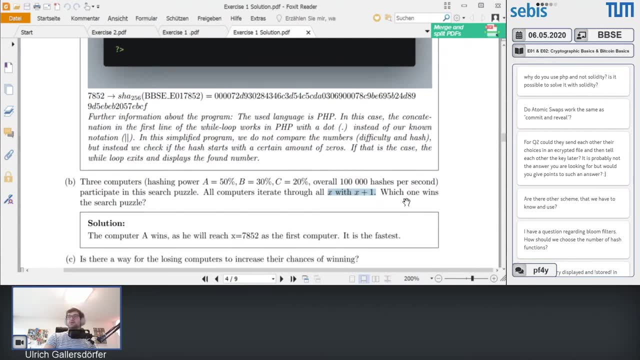 Possible participate in the search puzzle. all computers iterate through all the X with X plus one. So, like we do here, X is X plus one. um, uh, which one wins the search puzzle? So obviously The computer a wins as he will reach the solution. 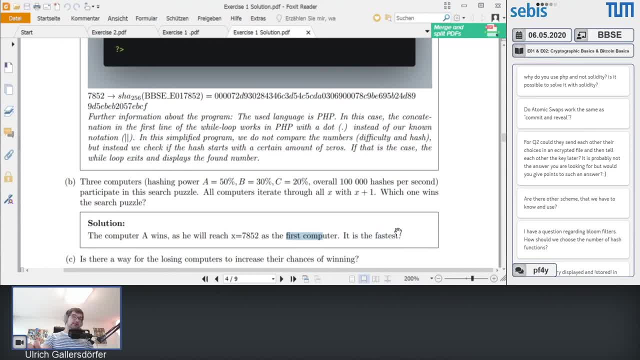 We calculate beforehand as the third computer, it is the fastest one, So that's for sure. the point here, Um, is there a way for the losing computers to increase their chances of winning? So that's a very good question. Can other people, other computers maybe, win in terms of, like their um hashing power? 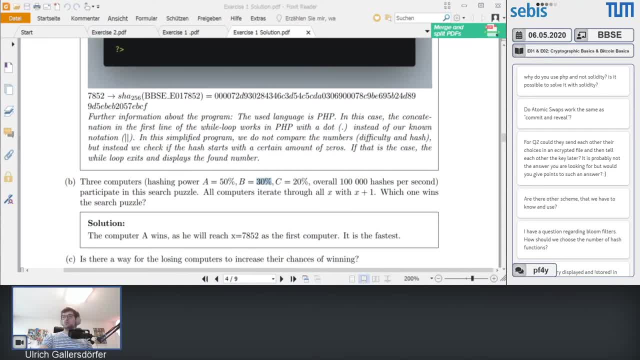 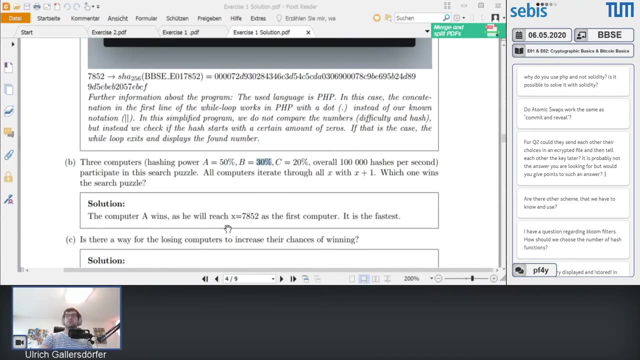 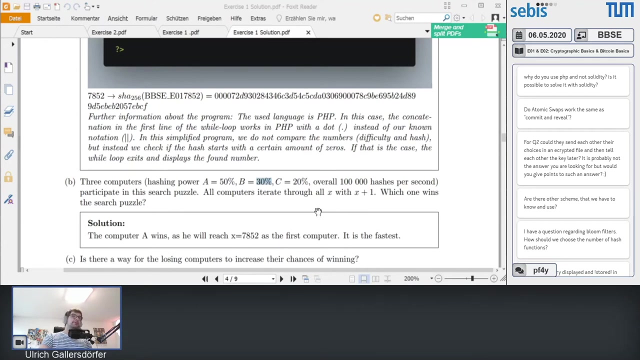 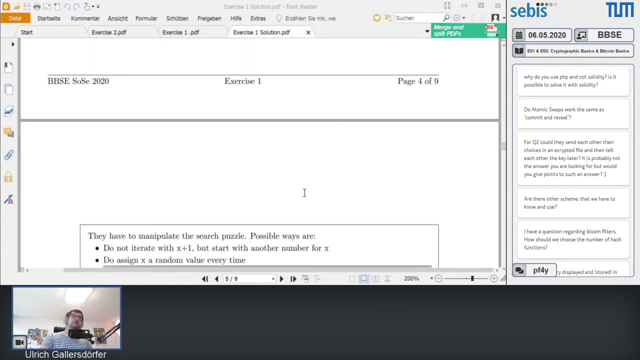 Um, so Um. the idea is here, um that We can increase the chances of the losing computers by um, not iterating through this, by X is equal to X plus one, but by selecting X randomly And um, this is. this is for the reason of the cryptographic hash function. 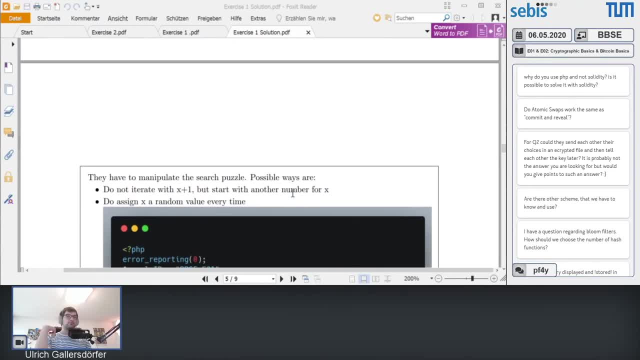 Because they um. the result of them is that the resulting hash function is like um, randomly distributed all over the output space. So we don't, we cannot um, um compute it. We, we cannot, um. how would you say it? 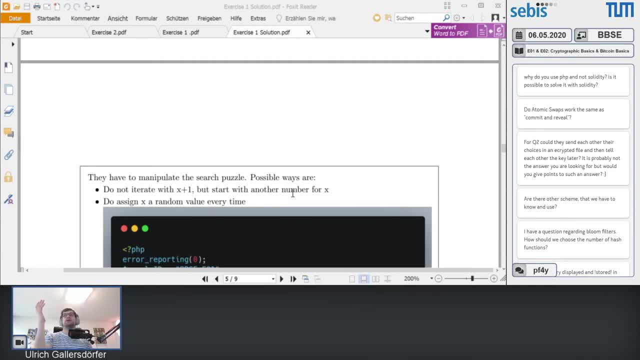 Um, we cannot, we cannot, we do not know the, the outcoming hash before we actually calculated it. So, um, taking random Um out of X, So um assigning random values to X, can be a bad approach than increasing from X plus um to to the next number, because then you have a, then you have a better chance. 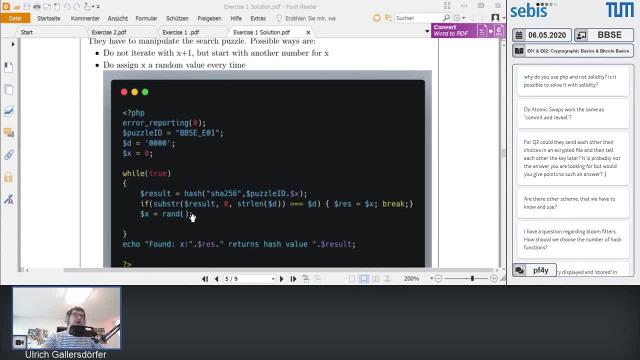 So you can try it out yourself um to take a rant here And um, then it's much more easier um to win this race, And if you simulate this yourself um- which we don't have time for um- you will. 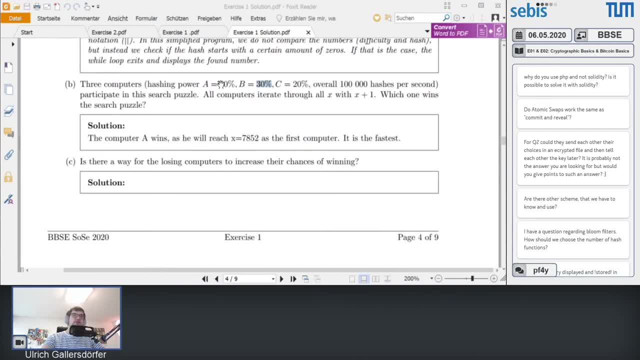 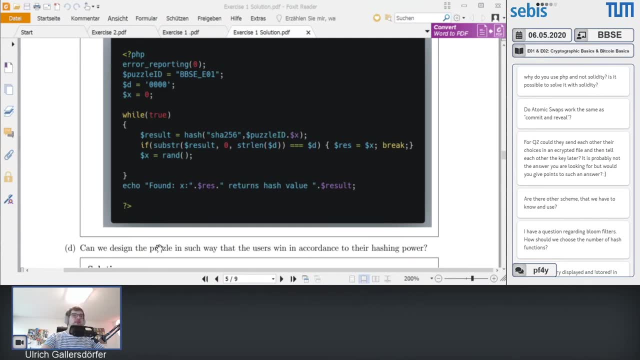 See that um in the long run, a wins with the 50%, B wins with 30% and C wins with 20% Um. can we design the puzzle in such a way that the users win in accordance to their hashing power? 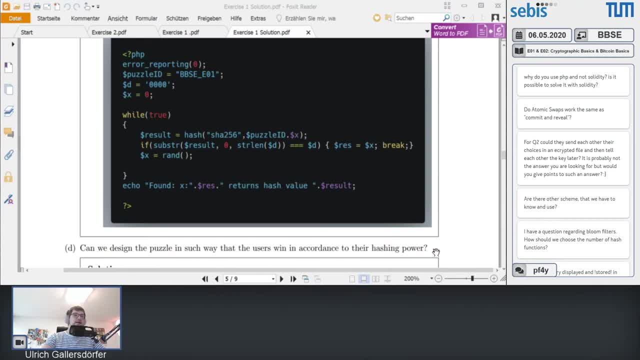 So now it's not the user in response to who's responsible for that, but it's the game designer, so to say, and we can do that. Um, it's not that difficult because we just introduce an additional Variable Um into that. 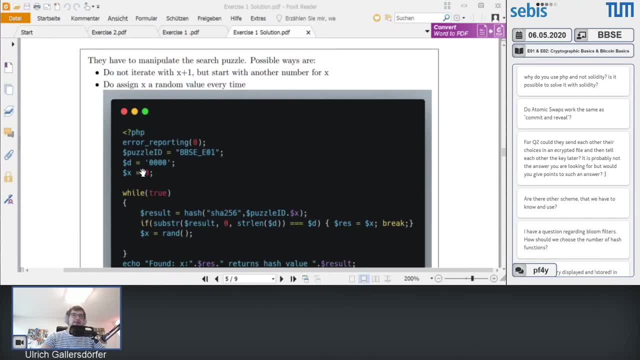 So we had the puzzle ID, we had the um X and now we can um attribute a user specific variable in there, For example the ID or the name of the player. And when we do that um, they can go back to iterating by adding plus one to X and it will remain um fair. 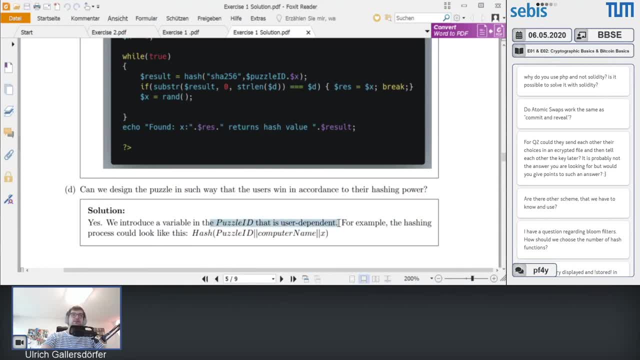 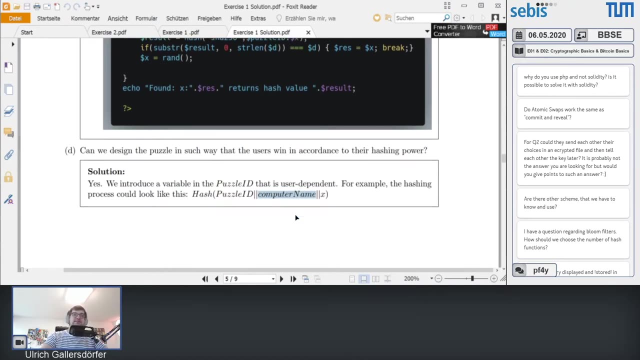 So we introduced a variable in the puzzle ID that is user dependent. For example, the hashing process could look like this: So the puzzle ID still remains in there, but we add the computer name and as this computer name is for um every participant different um, this um results in different hashes all the time. 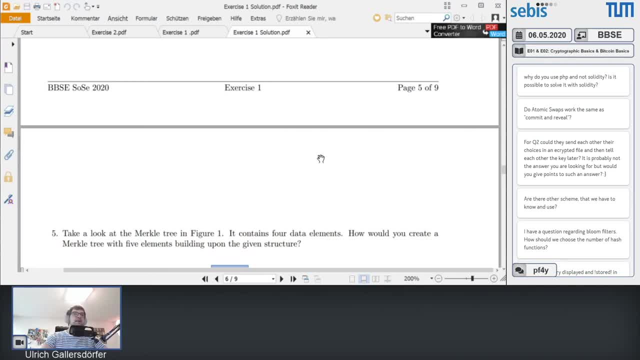 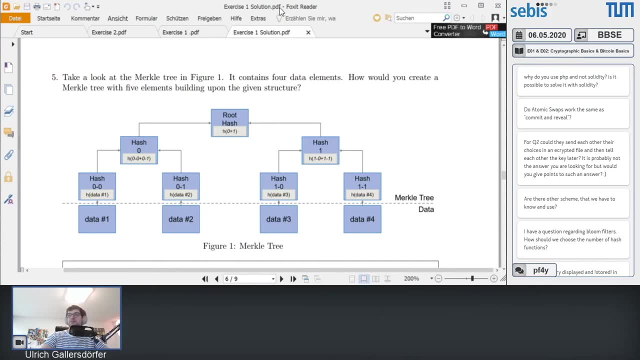 Okay, Let's take a look at the Merkle trees here. Um, we have these four data elements, So this is the Merkle tree we saw in um the lecture. Okay And um, I'm trying to okay. 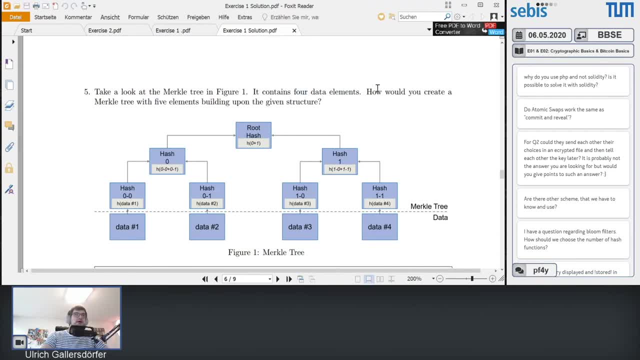 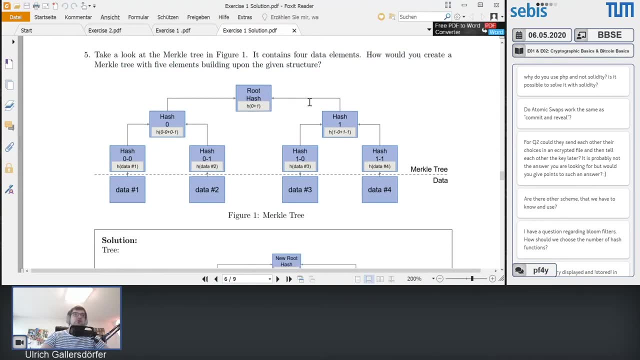 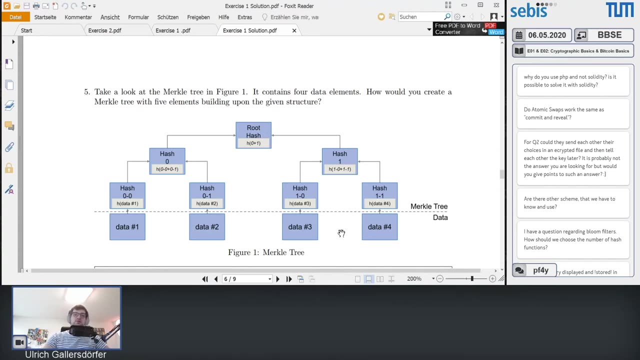 And it contains four data elements. How would you create a Merkle tree with five elements, building upon the given structure, Um. so the solution, basically, um can be, can be very, can be very different. So I have to say, and that's also what a lot of people ask, 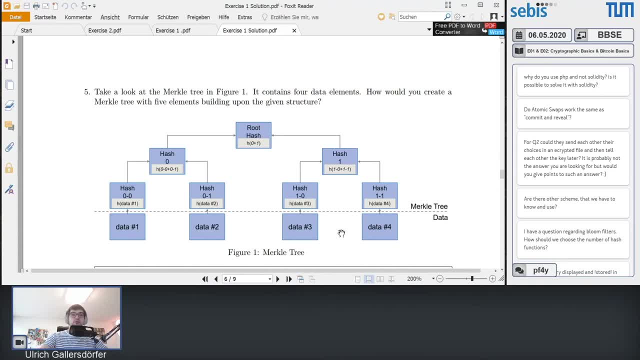 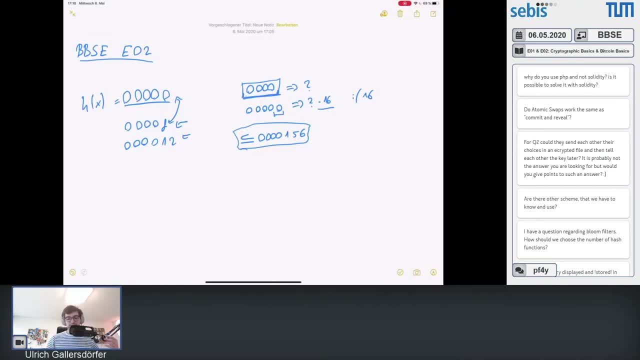 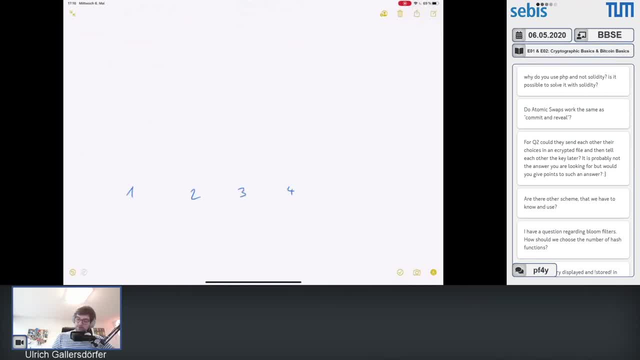 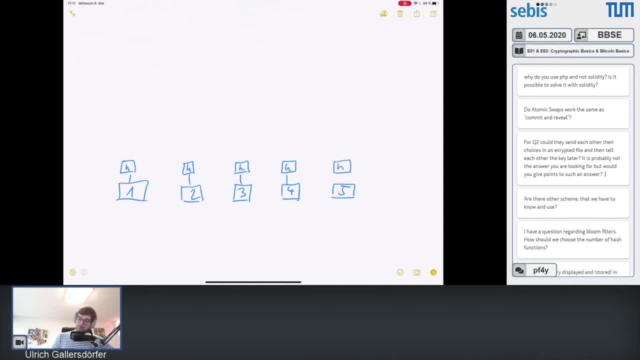 and we do a hash here, And that is fine. And now we need to concatenate hashes, So let's name it hash one, hash two, three, four and five. But what we do here is we create a new hash here and this hash is hash one I concatenated. 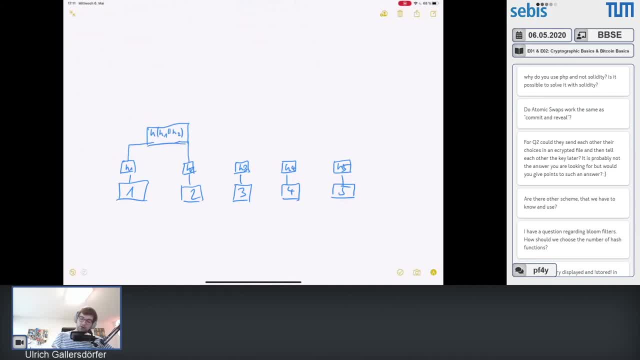 with hash two- This is also here- hash three and hash four. Now we approach this one here, this on the right, And that's not a good question, because there could be a lot of solutions in terms of, okay, we do something like this and now let's introduce that in here somehow. 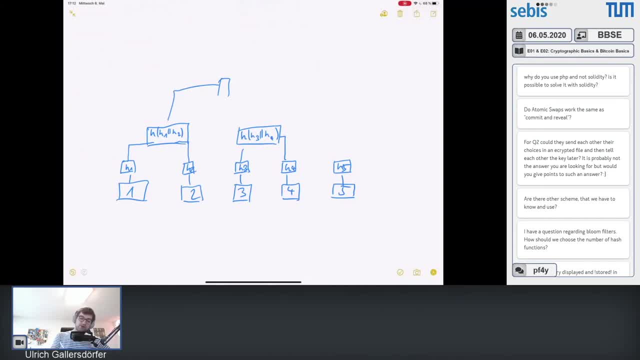 So that would work, but that's not really the official way. So I want to tell you how it's done in Bitcoin, because I think it's easier in terms of: okay, we want to do some kind of implementation. Okay, If we want to do inclusion proofs, we want to do that. then it's really equal for all. 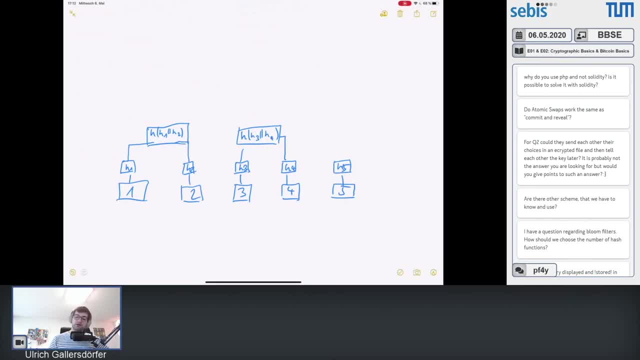 data elements. If you don't do that, you have a little bit of problem about that. So how Bitcoin does it in this case? if there is an element missing here, and that's currently the case- then it just replicates the element. 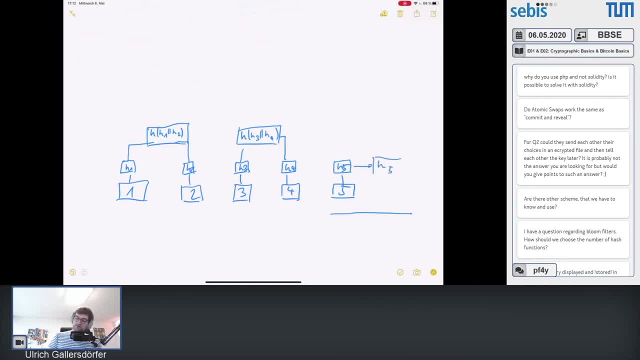 So what it does here is like: okay, let's just put H5.. Let's put H5 again there and do this as we did before. So now we have as hash from hash five concatenated with hash five, So now we can continue the same. 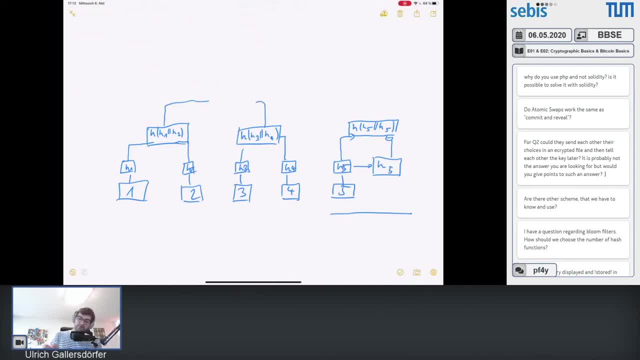 So this is again like this: is that's hash one, two, call it like that, That's hash three, four, And we hash hash one, two concatenated with hash three, four, And then we have this one covered. 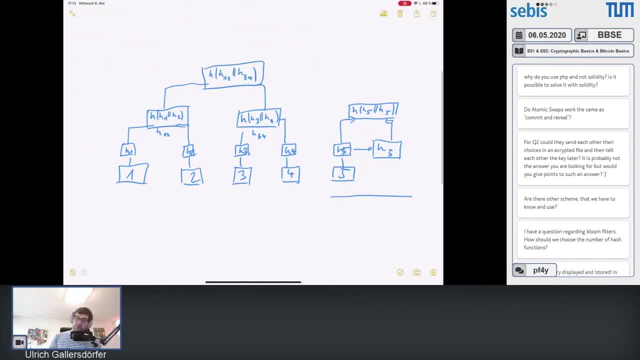 And then again we approach this here. So we now don't know how to handle this one, And this is exactly what we did again now. So this is replicated. this hash five five is again replicated to hash five five, And we do the same here. 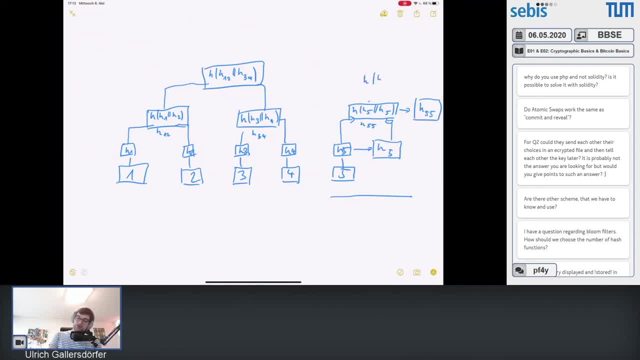 So we concatenate again the hash five five with the hash five five, And now we can calculate that. And now, finally, we have two elements left, and now we can calculate this root hash again by concatenating this hash and this hash. Oh, 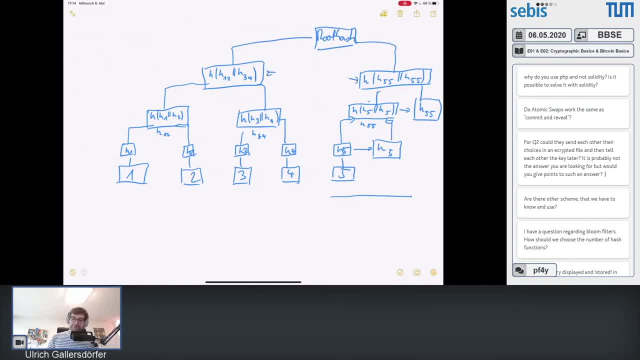 That one and that one, And so that's how you would add a fifth element in there. Also note that basically you can look here at the: So this one is our original tree And this is basically the second, the second half of it. 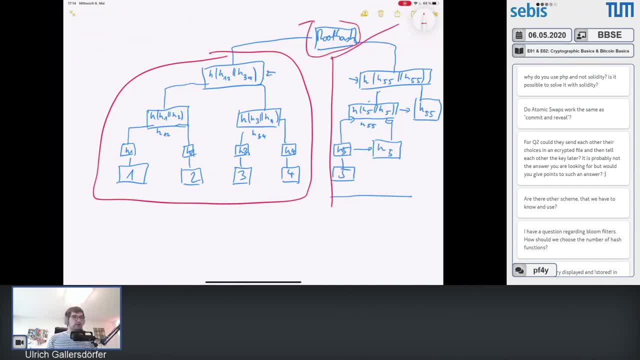 And this is the result, because we had some kind of an overflow. We have four elements there, which equals to three layers. So one, two, three And. but if we include more than that, then suddenly a layer zero arises. So that's the key point here. 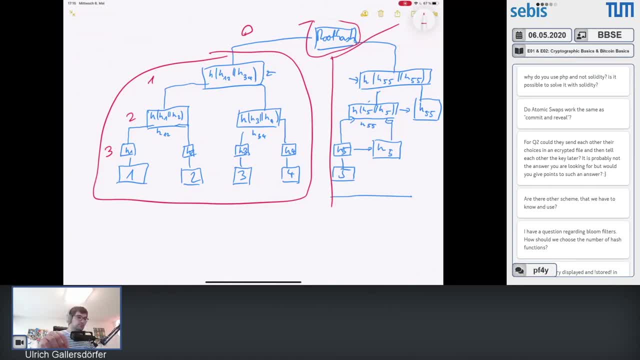 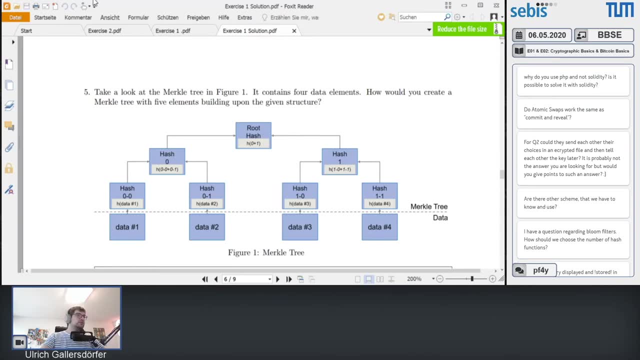 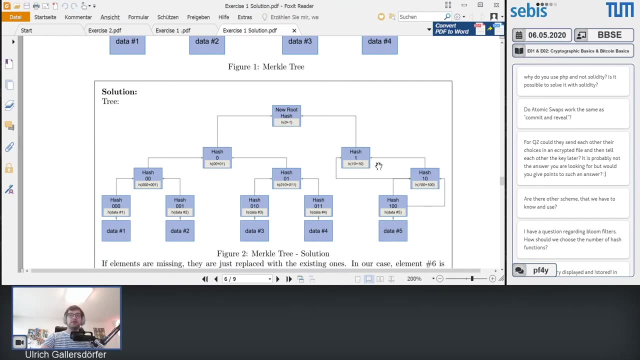 Okay, So let's continue here, Let's get back to our solution, And this is exactly what you will see here. So this is a little bit another display as I did it, But basically what we do is we duplicate the hash. If there is some element missing, we duplicate it there. 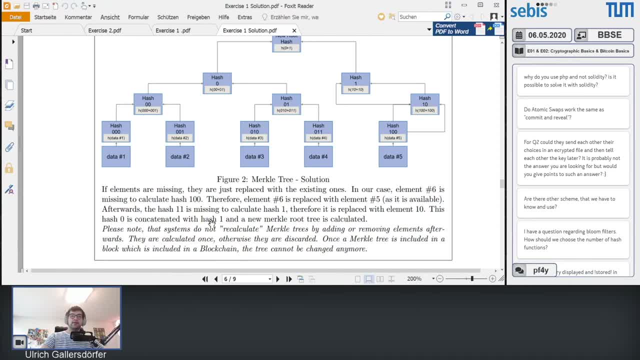 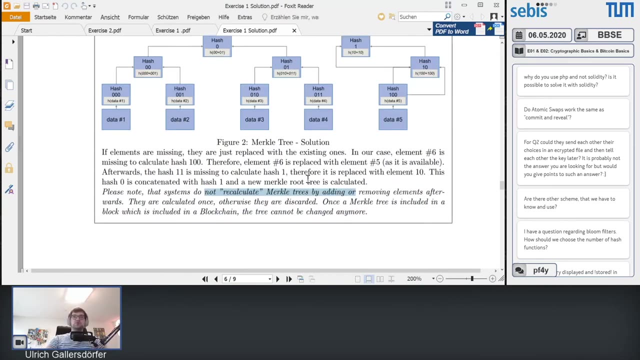 And also that's a very important remark here- Do not recalculate Merkle tree. So in blockchain You insert Merkle trees and, as the blockchain data structure is immutable by itself, That's very important- to that new trees are always added and never changed. 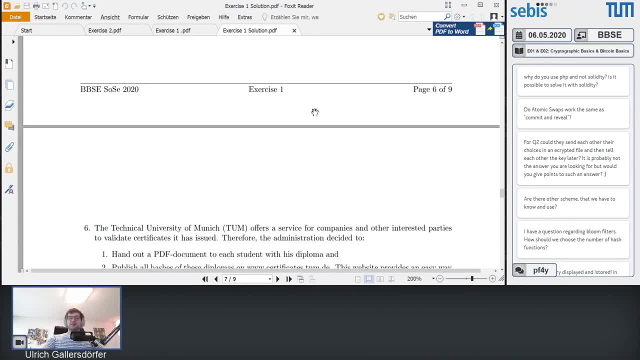 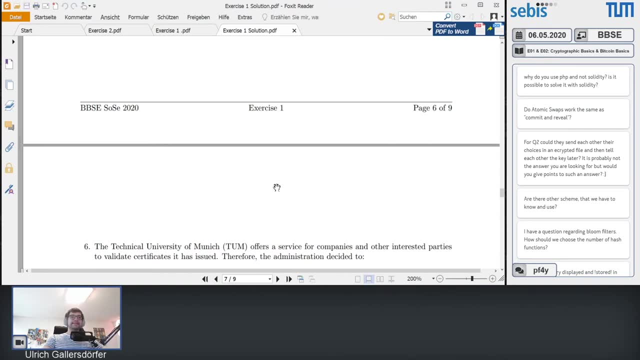 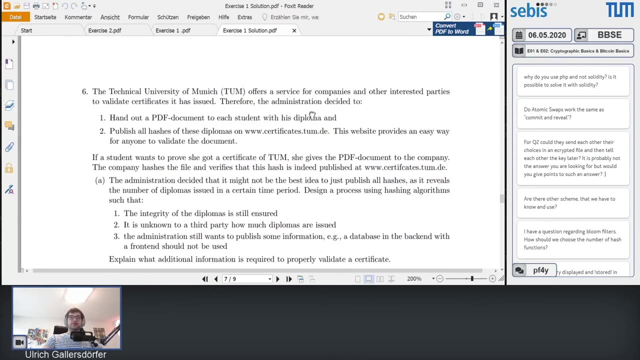 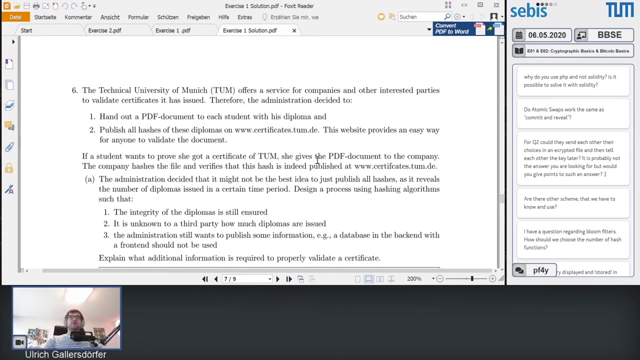 Okay, So the technical university. we have a little bit on timing issue. Sorry, I spent too much time on the first part And so the Let's take a look at this question here. So the technical university of Munich offers a service for companies and other interested parties to validate certificates. 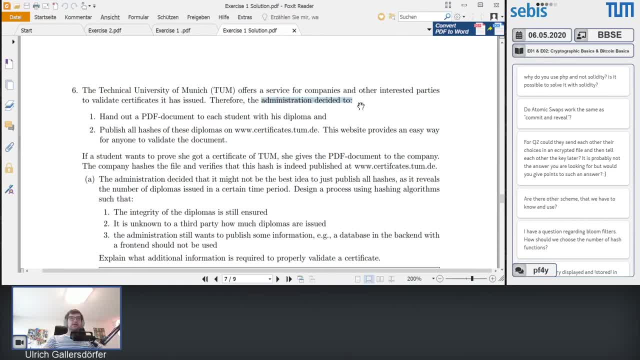 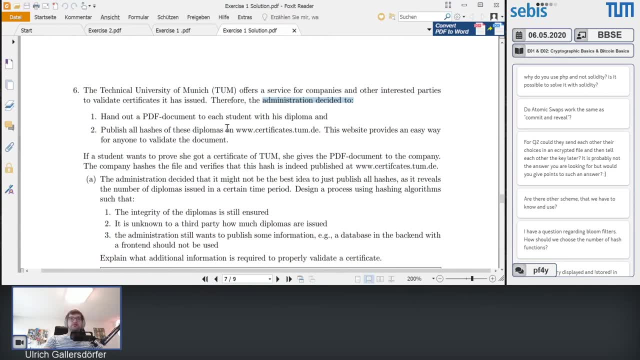 Is has issued. Therefore, the administration decided to hand out a PDF document to students with his or her diploma and publish all hashes of these diplomas on certificates To This website provides an easy way for anyone to value validate the document. Okay. 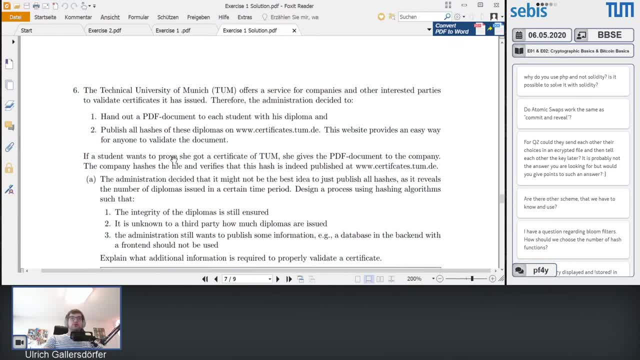 So if a student wants to prove she or he got the certificate of whom, she gives the PDF document to the company. the company hashes the file and verifies that this hash is indeed published at certificates To Te Hey. the administration decides that it's might not be the best idea to just publish all hashes, as it reveals the number of diplomas issued in a certain time period. 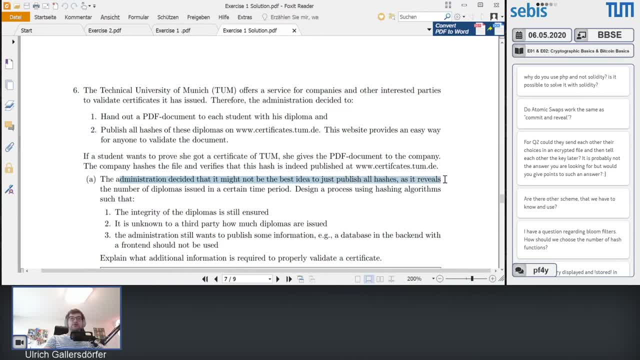 Design a process that allows you to publish all hashes. So that's the first step. Okay, So this is the first step. So the first step is to design a process using hashing algorithms such that the integrity of the diplomas is still insured. 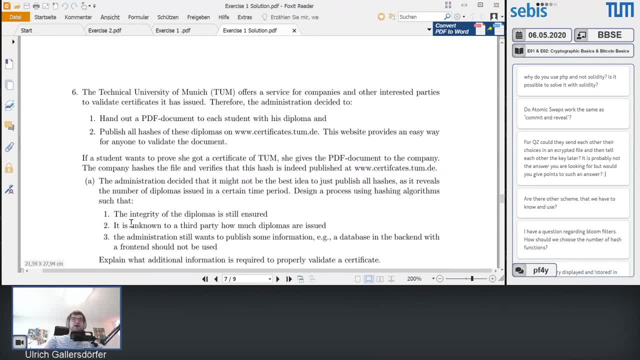 It is unknown to a third party how much diplomas are issued and the administration still wants to publish some information Each year. database in the back end with a front end Could not be used. Explain what additional information is required to properly validate a certificate. 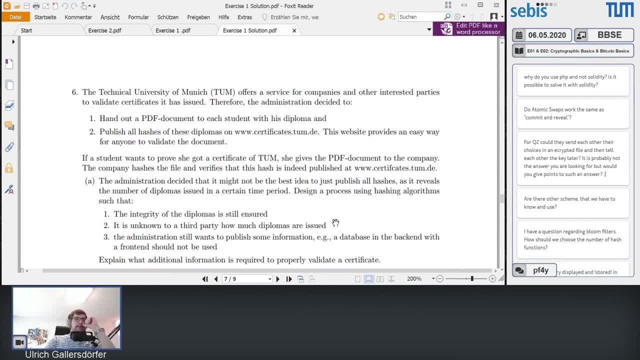 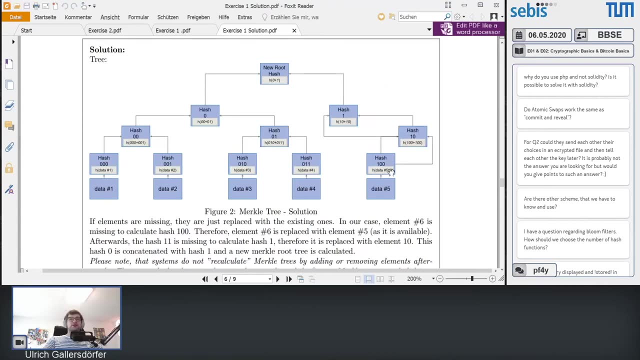 So That's Uh Uh. The basic idea here is To say, okay, as we introduced it in the lecture, we want to use Merkel trees. So we saw that beforehand how we set up a Merkel tree, how the status structure looks like. 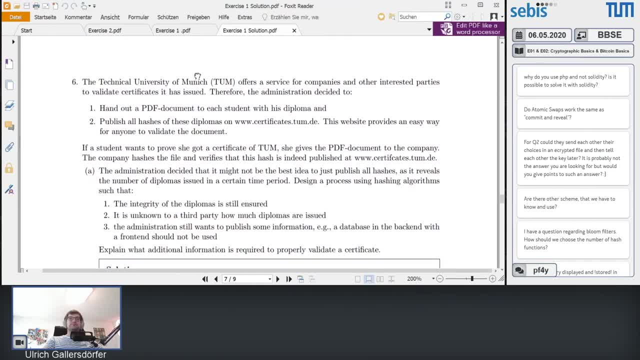 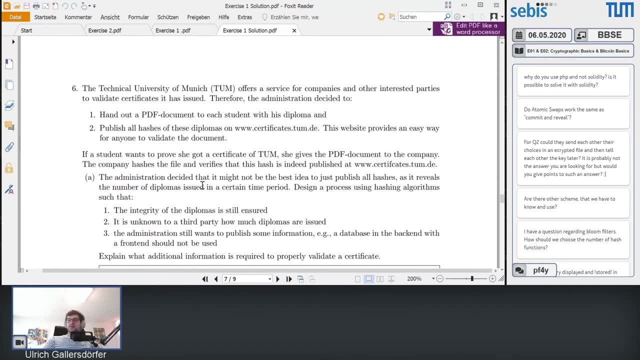 And what we can do now is we can Also create for the TuM a Merkel tree, So, for example, the semester ends and 200 people graduated, And then all these Hashes of these 200 documents can be stored in one single Merkel tree. 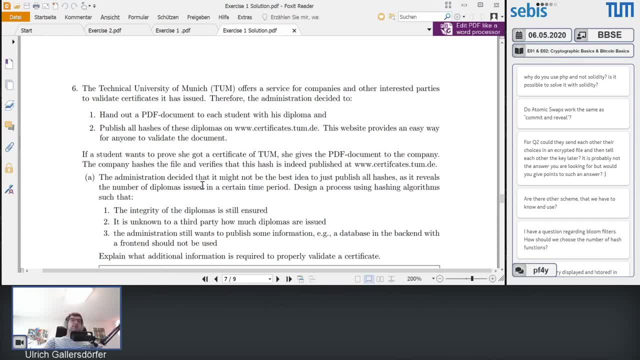 And this hash, the root hash of the Merkel tree, can be published to um. these um certificates, TuM, Um, but unfortunately you need some additional um information if you want to use um Merkel tree And um. that is basically the um membership. 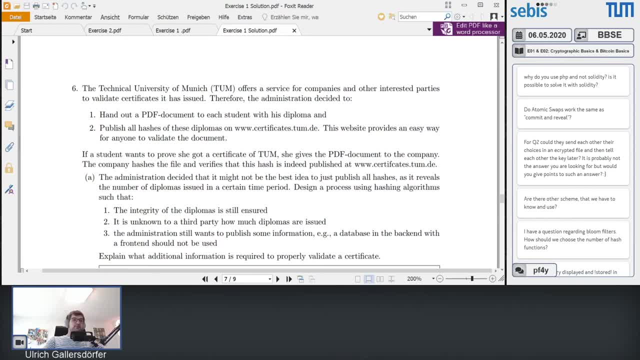 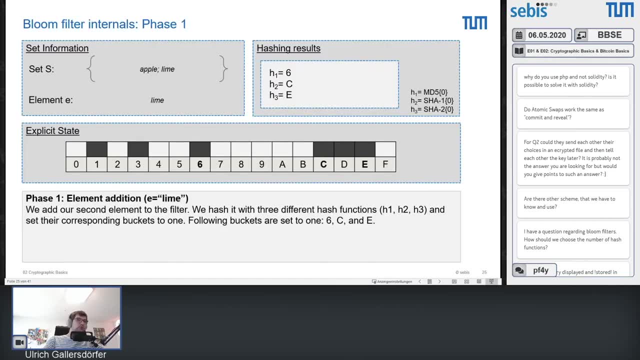 Um proof. So, as you remember from the PowerPoint slides, Let me see if I have them here. Um, Yes, I have them here. If you remember, Uh, This one, this slide, Um, you basically need to provide this information, um alongside the um certificate, such that. 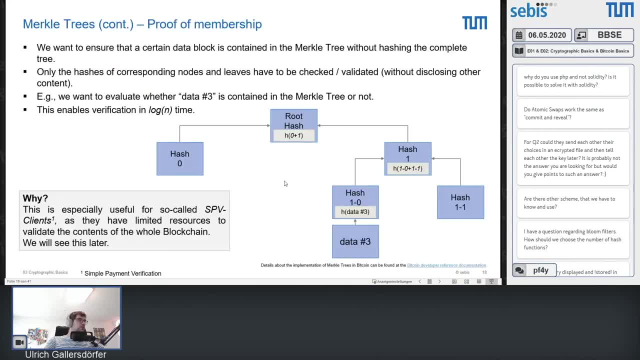 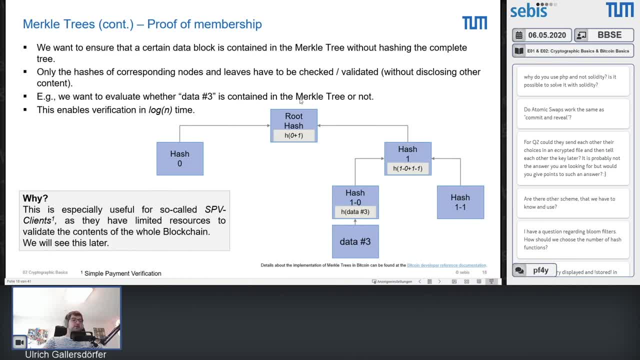 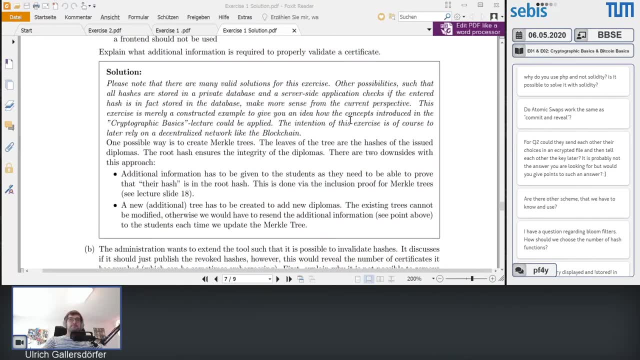 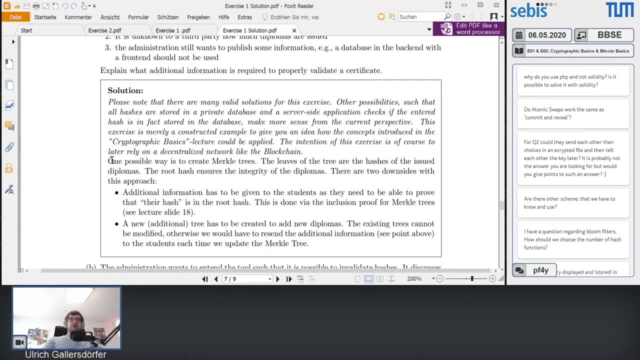 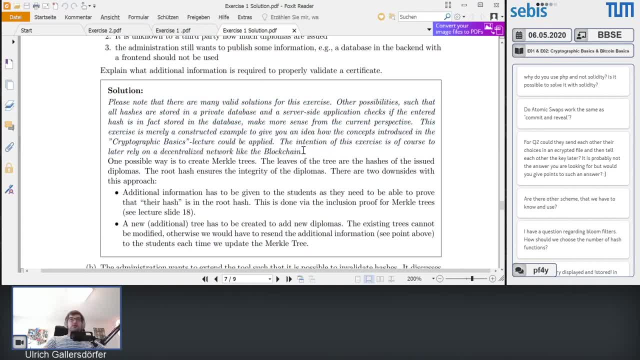 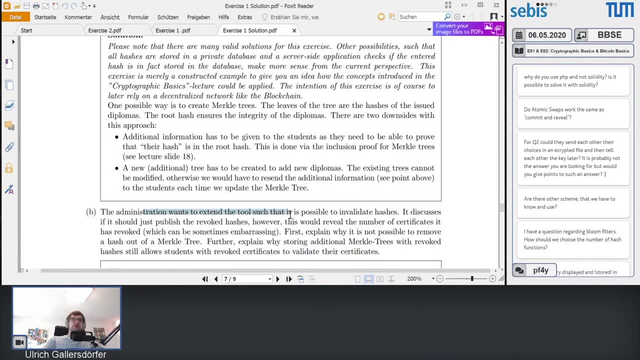 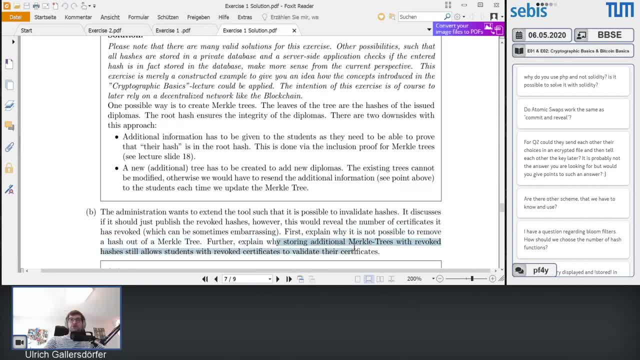 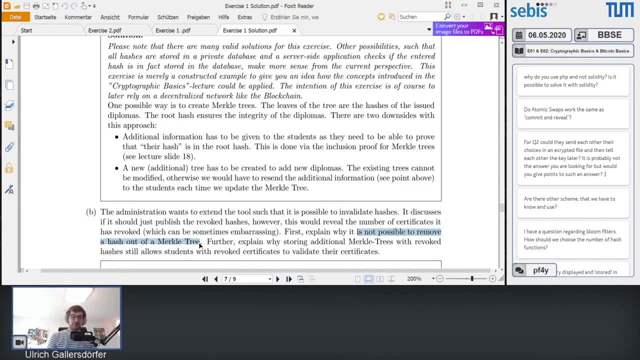 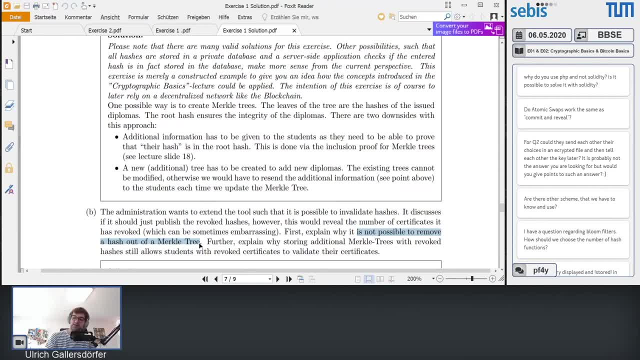 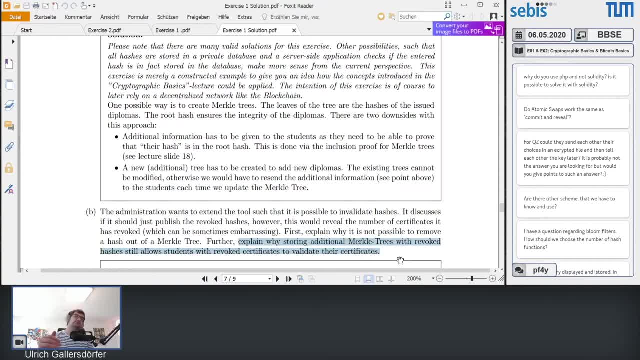 This is also an interesting point. If you would basically also publish Merkle trees with revoked certificates, then there is a downside to that or it would not work, Why You would have to provide this proof of membership to the student who has his certificate revoked. 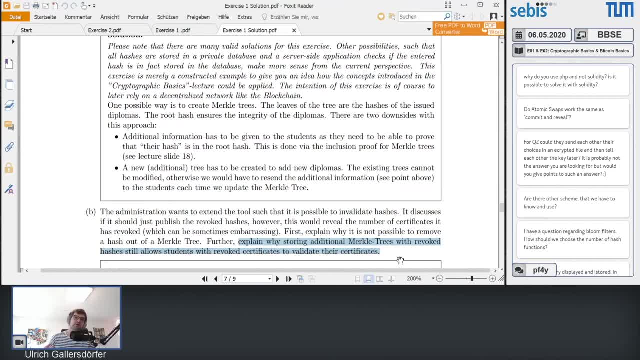 This student could just omit this information and say, okay, I'm not giving this out to another party. The third party would have no way to check if it's actually in the Merkle tree or not. That's the reason why we cannot use Merkle trees for revocation purposes. 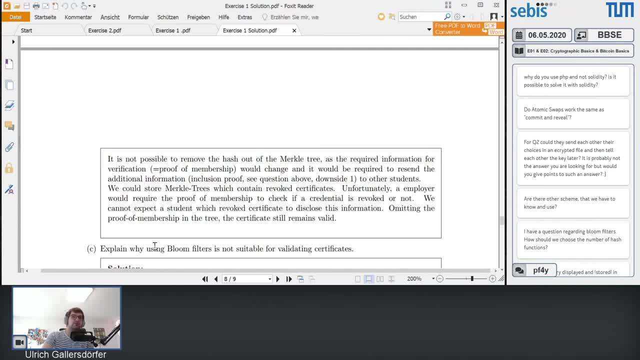 That's also in here. Thank you, Explain why using Bloom filters is not suitable for validating certificates. but that's the membership question again. Bloom filters would be a very nice idea but, as you, as I told you beforehand, the Bloom filters itself are not suitable because it is very easy to generate. 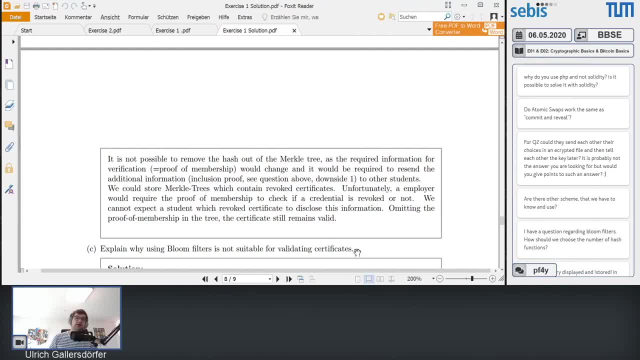 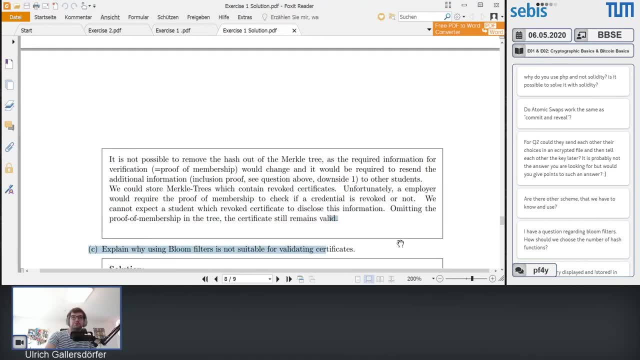 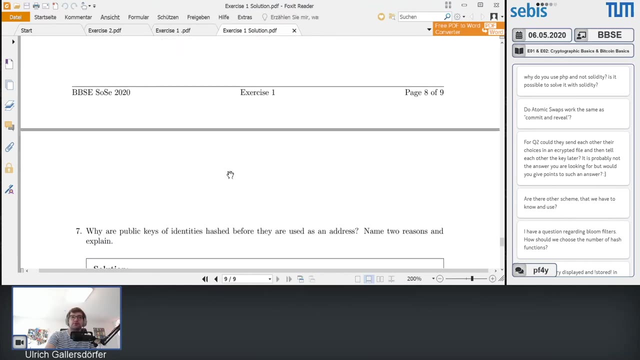 false positives, or it's likely that false positives occur And with that you could basically fake certificates. So it would be not a very good way, Yeah, Okay, Let's move to the last question, And the last question is about public keys of identities.